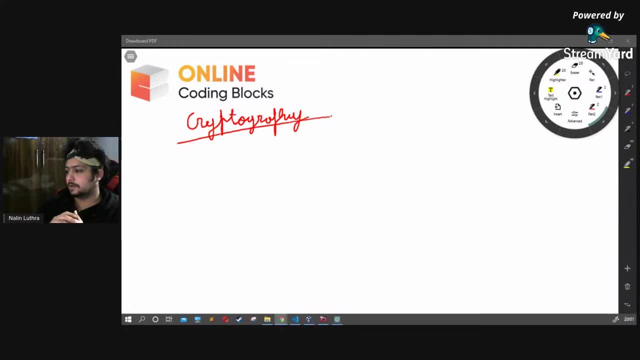 on it. We're going to start today Everything. So good evening everyone. I know many of you are already having some doubts at where I was, what I was doing and stuff like that. I completely agree with you. But yeah, I had a busy week, So yeah, So I guess everyone enjoyed their. What are we talking about? I have no clue about that, So I think you should listen to Scott. Someone will take up that doubt. I don't know what you're talking about. Happy New Year guys. Happy New Year. Happy New Year. 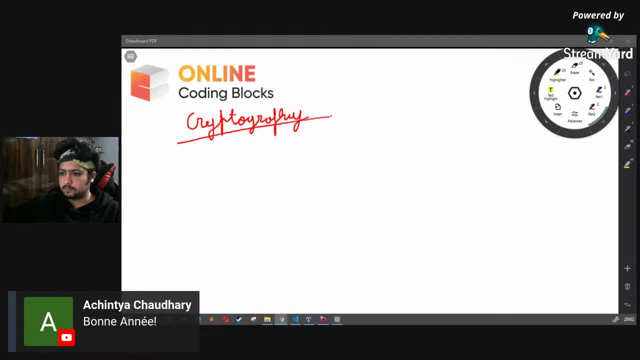 Happy New Year. I don't know what this means, I don't know. Maybe same to you, I don't know. If it's good, it's good, Okay. So I think everyone is good right. So I know it has been at some time. I got, Yeah, Thank you so much. Thank you, Yeah. So I had, But in my weekend, like last week, I had a birthday, So I was busy with that, Enjoying and stuff like that. Okay, Yeah. 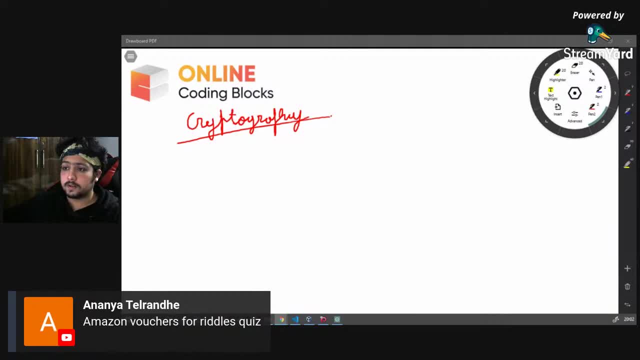 I don't know. Okay, I will confirm about it. I will give you an update on it. I have no clue personally. I have to figure it out. I don't know. This is on Discord, maybe, Okay, Okay, Hey, Abhinav, I know you're new here. That sounds good, man. So today we're talking about cryptography. today, So it's a topic of hacking and it's a cyber security. let's say that. So we'll talk about cyber security and everything in this lecture series. So, hey, Abhinav, Welcome. 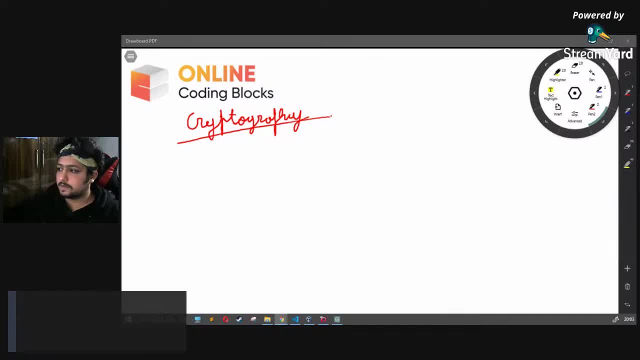 Let's start and see how it goes. Thank you so much, guys. Thank you so much. Yeah, We got the message, man, So honestly, Okay, Happy New Year, Happy New to you. Okay, I think everyone is good now. Okay, So it's like it's We're taking clusters for so long, So let's wait for a couple of minutes. Let everyone join. If anyone got some doubts on anything, let's pick up that I don't know. Let's move forward, Okay. 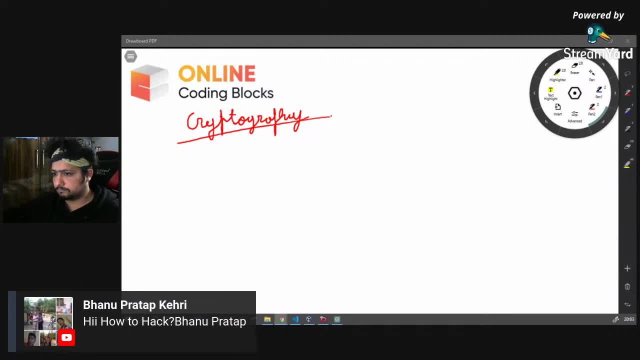 Okay, Yeah, It's good if you have a decent knowledge about Python, because today we'll start programming on Python, because I plan to actually start programming tomorrow. But a lot of you guys are quite curious to know how to program, how to write codes and cyber security and everything. So we'll start with it today. So we won't take the blame for tomorrow. We will do it right now, right here, with everyone else, So it will be cool. 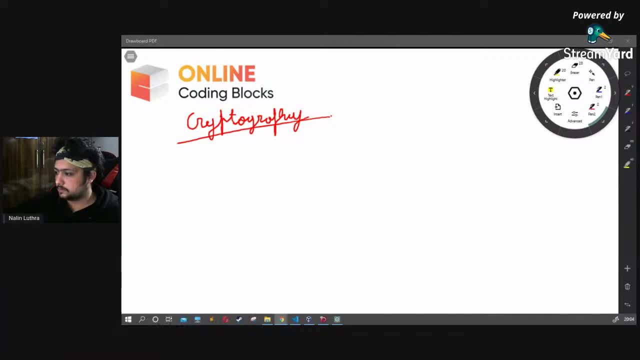 Yeah, That's what I use. That's right, That's what I use. Oh, school class is a bit strange. No, it's not a school class, man, It's not a school class. Don't say it's a school class. 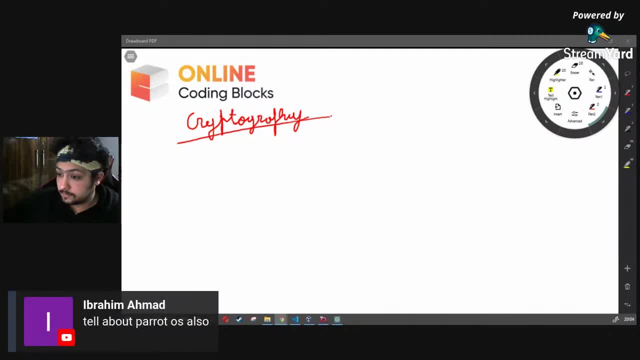 Oh yeah, That's it Okay. So don't think about operating system. right now. You use Ubuntu, Linux, Sorry, Ubuntu, Kali Windows, Mac Parrot, It doesn't matter. This is Anurag. I will try to do it. I cannot assure you about that. First of all, it's just a lot of things are going on these days, A lot of I don't know. I don't have enough time about this, So we'll figure it out, So anyhow. But yeah, definitely we're going to have classes on weekends, Don't worry about that. So I know the last couple of weekends wasn't busy for me, So that's why it got somewhere out. But yeah, we'll work on it. 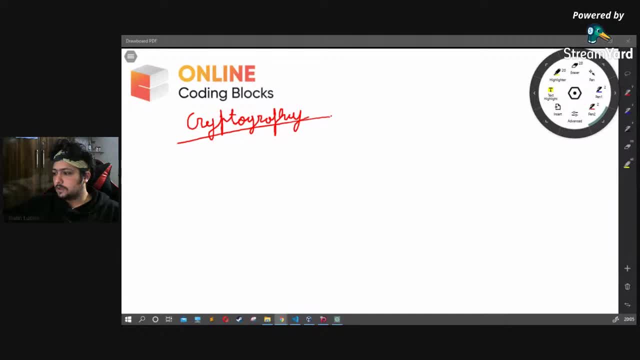 So, yeah, you will have classes. Okay, So, let's start for today. Yeah, So, everyone is here. I think we should start for today itself. Don't forget to like, subscribe and share. I think that's where we say it at the end, So, yeah, So let's have a drumroll and start with today's lecture on cryptography. I don't know, It's weird. Okay So, Alexa, drumroll please. 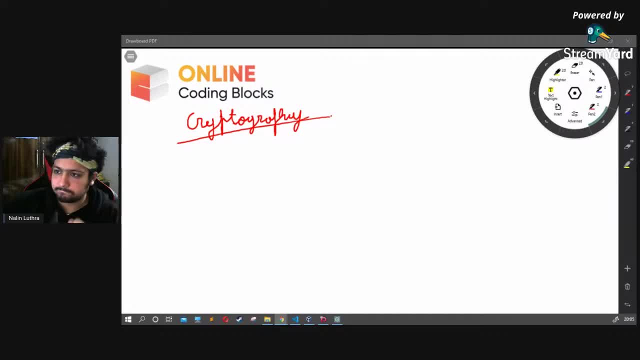 Okay, All right. So today we are talking about cryptography, So cryptography is one of the most important branch in hacking, So there's multiple reasons why this branch is extremely interesting, important and slightly mathematical. Let's understand from the basic itself. So why I'm saying the cryptography is interesting, even though many people think cryptography is boring. 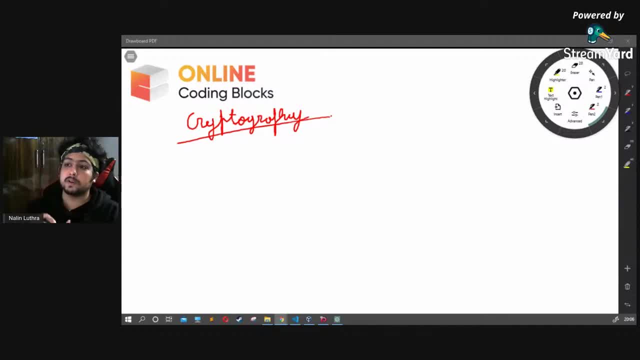 Because that's not what. something looks cool to every one of us. But cryptography is really important. Our whole world, whole society right now is completely indulged and is working only on the basis of cryptography. For example, you make a bank transaction, So every data has been transmitted using cryptography, right? So if there's no cryptography, there's no encodings and everything, So we will transfer data. So let's understand how cryptography goes. 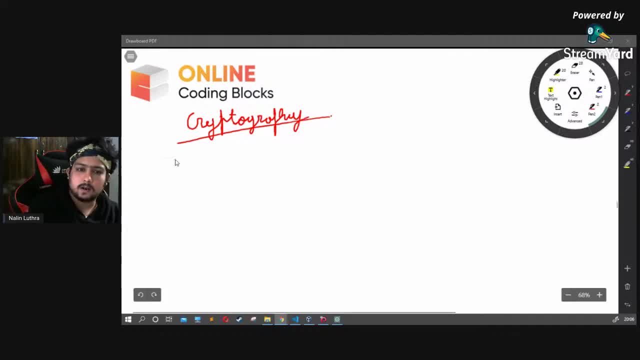 Okay. So let's say, over here I have an engine. Okay, So let's say, I got an engine with me. This is a function. Okay. So this is a function which encrypts whatever I give. So, for example, let's like this: I write A and output: I get C. Okay, I write B and output- I get D. Right, So that's how it goes. So this is a function. Let's say it's a cryptography function. 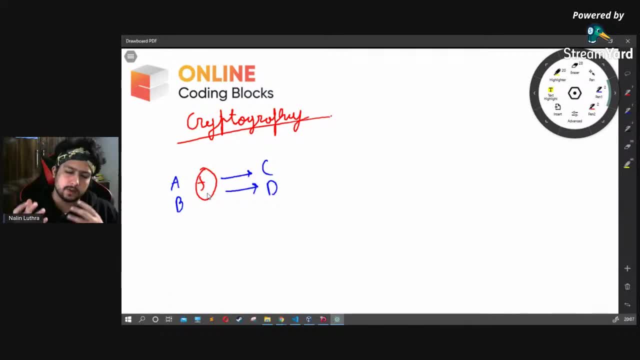 Or a cipher, So these are called ciphers basically. So we will talk about in depth. So this is a basic understanding of the whole scene. Okay, So let's say we got, say A, we get C, we get B, we get D. So if I say A, B, B, B, A, B, B, A, Right, So what output would I get? I would get CD, DD, CD DD. 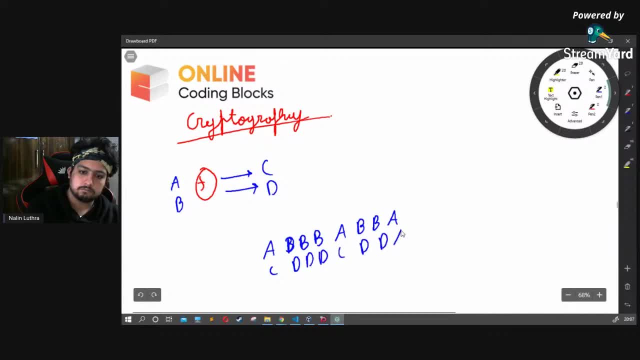 Right, That's simple. So these are ciphers. When you convert from A something to something else which cannot be read by humans or anyone else altogether, That's how ciphers work. So ciphers are not what like. it's not starting from today itself. Ciphers are there from since beginning. I would say It's been a long time, Every single, when kings and queens were there. 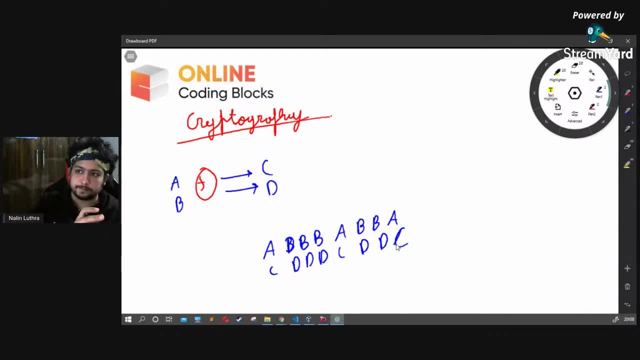 But they also use ciphers to transfer data from one area to another. Okay, So when we talk about hacking and cybersecurity, even the people like us altogether use cryptography to send messages on WhatsApp, because WhatsApp are two way encrypted. We'll talk about that in a while. So that's how it goes. So that's what encryption or cryptography in basic and overlooked means. So I'm going to leave it to everyone, Like everyone understands what cryptography in a really basic way goes like. 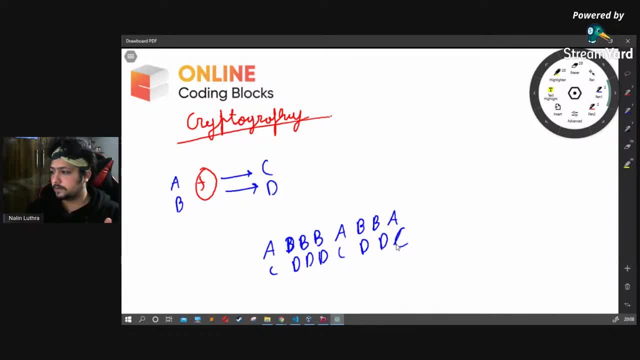 Okay, Someone is saying: please talk in Hindi. Okay, My Hindi is bad, guys. I guess you guys know all about this already. Okay, So Hindi is something that turns your written words into other words, And that's cryptography. That's a pretty obvious Right Cool. So, guys, moving forward. 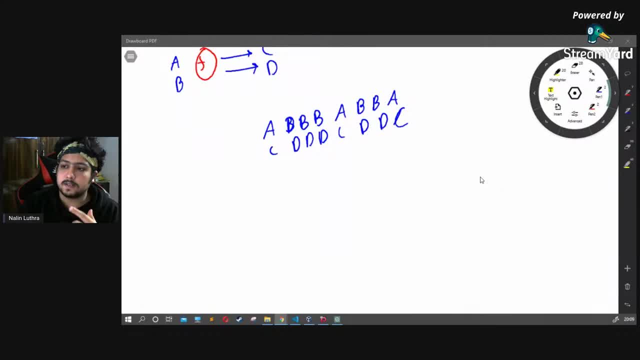 Okay, We'll talk about two cryptographic algorithms. One is Caesar cipher and other is monosubstitutions. That's the two we'll talk about. We'll write code on that and Python as well today, So that's going to move forward with that. 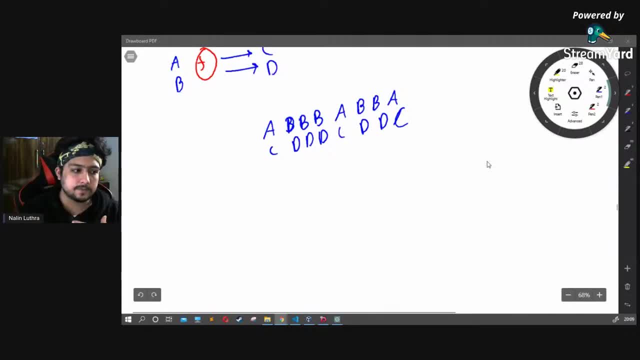 Okay, So let's understand what are different types of cryptographies. Let's take to that one. I think I have space for that. Okay, Let's draw a line and talk about types of different cryptography. Okay, So we have Cryptography. I don't know how I should. Should I do cryptography? Let's call it C like this, So that would be more interesting. 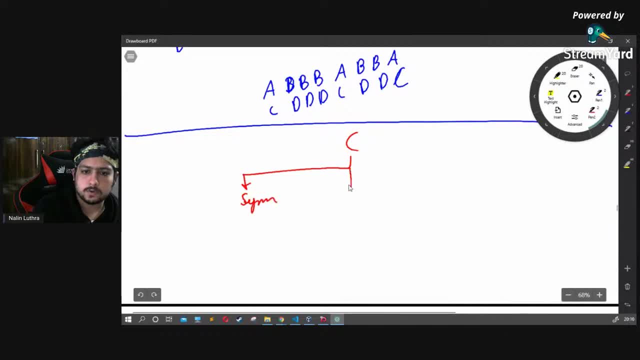 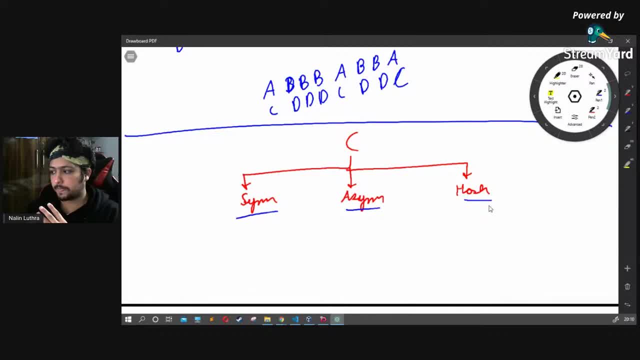 Okay, One is symmetric. Okay, One is asymmetric. Okay, One is asymmetric. Okay, One is asymmetric And one is hash. Okay, I don't know what people are saying. Okay, Okay, Guys, if something you don't understand and I'm speaking too much in English, just ping me that I should say the same things in Hindi as well. 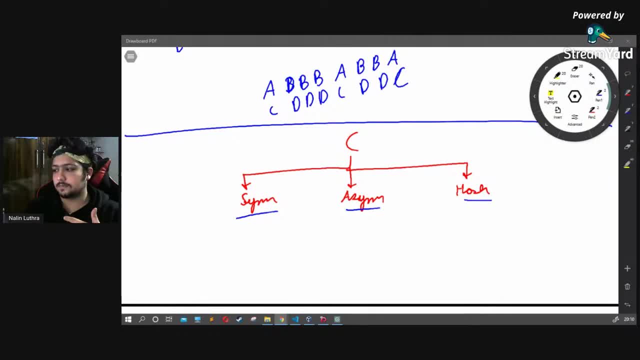 Because my Hindi is not that good. Even Hindi is not that good, So I don't know. But whatever, Move forward. Okay, So we have symmetric, asymmetric and hash. Okay, We have three different ways of saying it. I don't even know how to say it in Hindi, so I won't be able to tell you anything. 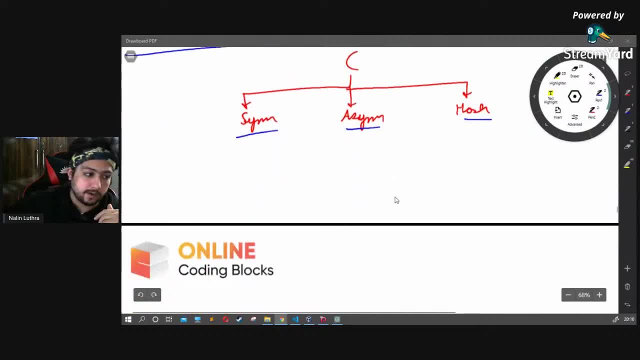 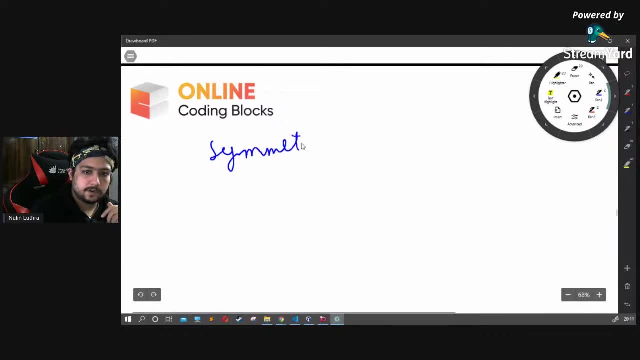 So what exactly symmetric means? So let's first pick up the point of symmetric. Okay, So we have symmetric. In case of symmetric, it's quite simple. I know right, I know. I will not try to talk in Hindi. 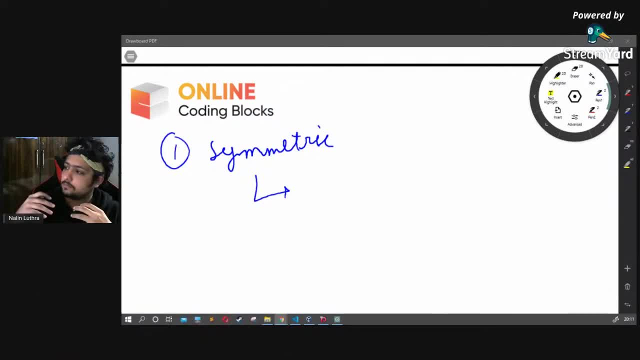 Yeah, Okay, So Okay, Mixed language is fine. Let's figure it out. Let's move forward slowly. I don't know why people are writing FFM. What does that mean? Okay, So symmetric, So symmetric cryptography is basically when we have a same key for the encryption as well as decryption. 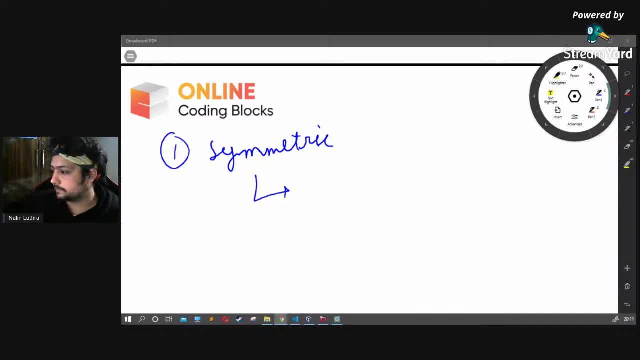 Okay, So let's understand what is encryption and what is decryption. We will talk about that in the future lectures itself, Or maybe today itself- Let's see how much time we have for that. So we'll talk about that, Don't you worry. 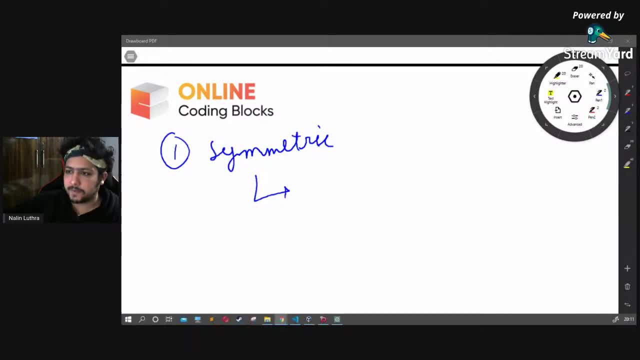 Okay. So let's move forward slowly. Let's understand the basic concepts before moving too much fast and not able to grasp what was actually the thing behind it. So let's talk about it slowly, Okay, Okay. So just giving you a basic idea. 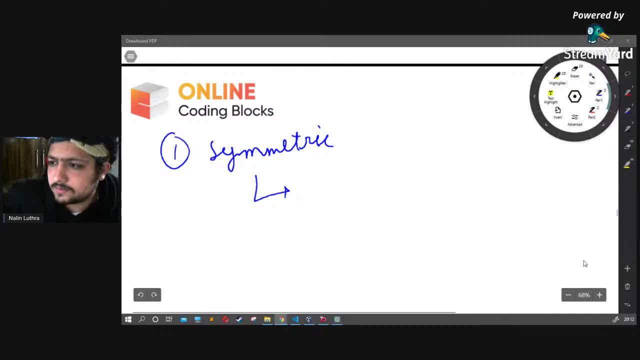 Two-way encryption works on asymmetric transactions. Okay, We'll talk about that, Don't worry. So we have symmetric encryption. So what exactly symmetric means? It means that when we call about two-way encryption, okay, let's say we have encryption and we have decryption. 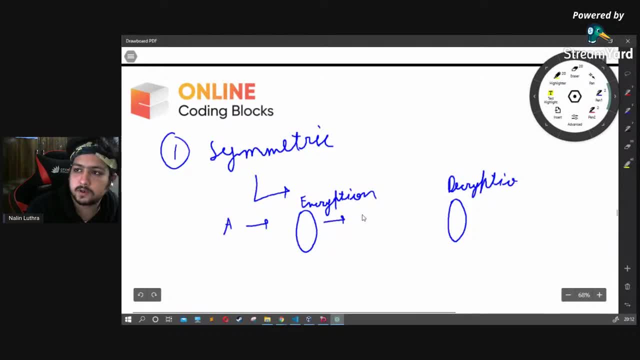 So, for example, if I send A, it gets converted to I don't know 1. And in decryption it gets converted back to A Right. So over here, this area is the channel of transmission. Okay, Transmission. 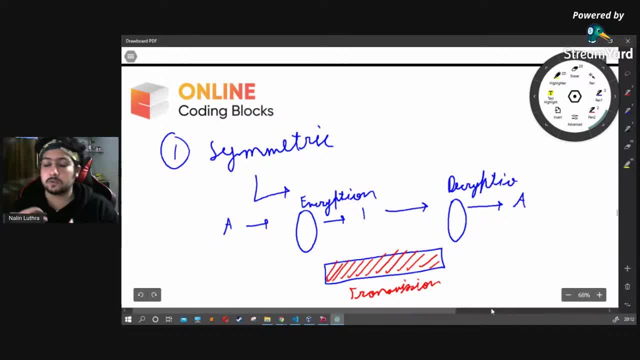 Okay So let's try to understand this a little more clearly. Think like this guys: Okay So I'll tell you a little in Hindi. Let's talk in Hindi for a while. Yes, Today we'll do practical. It's been a long time. 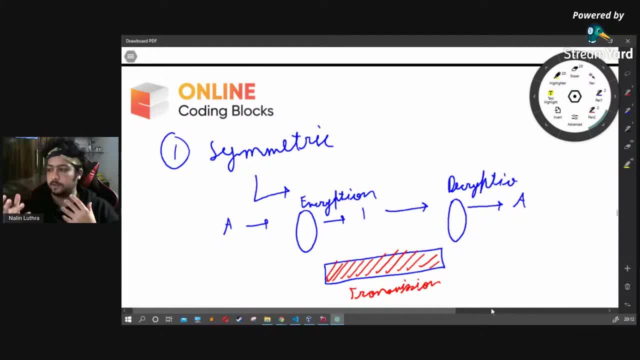 We haven't done practical. I mean, we don't do code Today. we'll do code, We'll write some good code And you'll have to hack that code. Okay, Okay, Okay, Okay, Okay, Okay Okay. 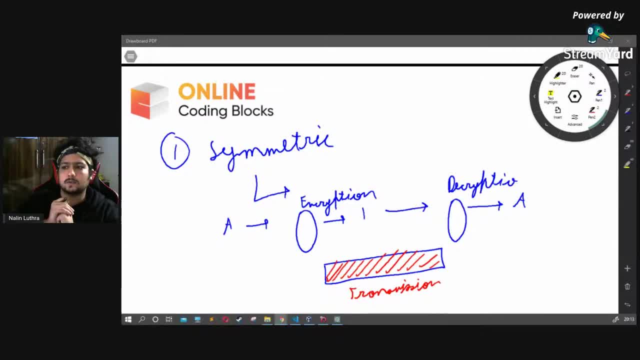 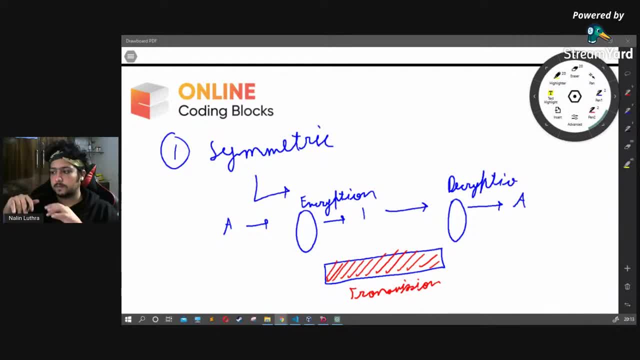 Like if I talk about the internet, what I am saying I am typing here I am sending a message from one person to another Means I am sending a message from here to there, So that message gets transmitted from many places in between, right? 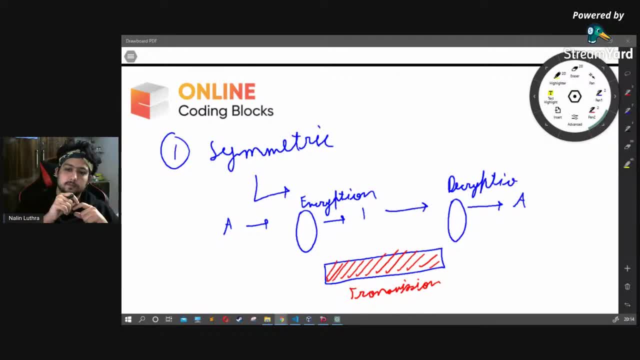 At that time many people can read that message. To save that thing, we encrypt it. So, for example, I am giving A By encrypting A, I have done 1.. Now, where will it be to do A again? 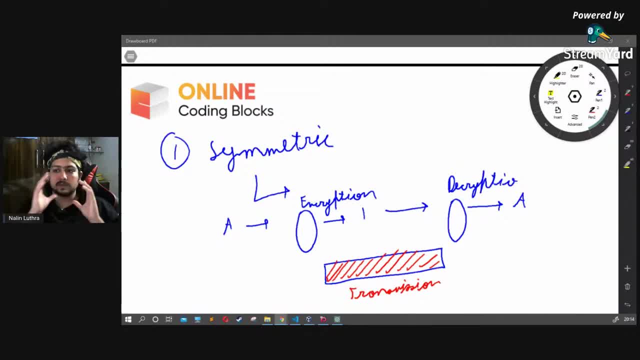 Where it has to deliver the message. So that's how it goes with encryption as well as decryption. So A gets converted to 1 and 1 gets converted to A, back to back. So this is what is called a symmetric. 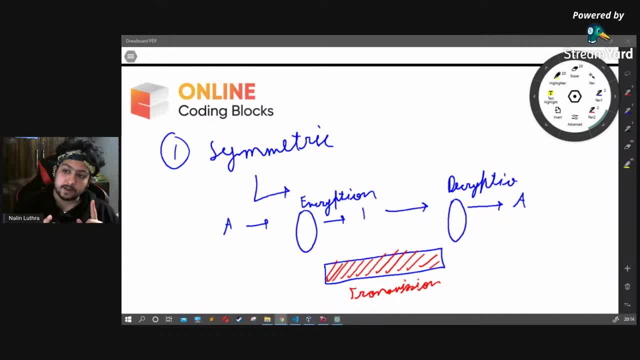 Okay, this is not symmetric. This is basically just encryption and decryption, But when we use same key for encryption as well as decryption, it is called symmetric cryptography. Symmetric key cryptography Is everything clear If I am using the same key to encrypt it. 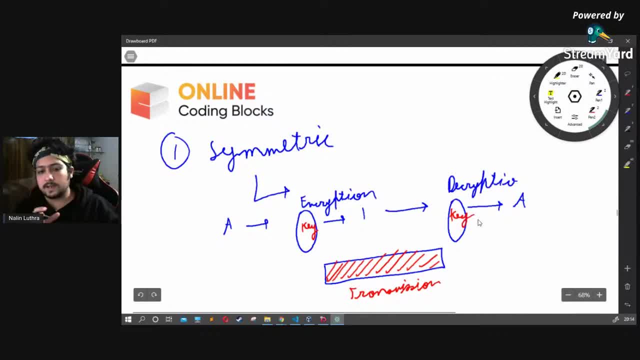 and I am using the same key to decrypt it Means to use the same key to encrypt it and to decrypt it. you will say symmetric Means whatever key I have. Okay, I don't know, this is weird. Maybe like this something. 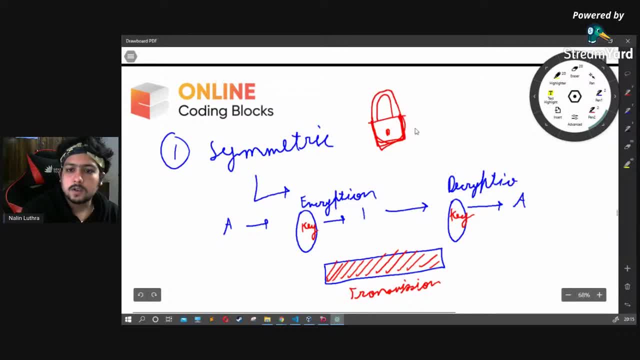 Yeah, This is cool. Cool, So I have a key. Okay, Let me find something small, Cool, All right, Cool, Let's add something like this: Cool, So I have a key. Okay, I am using this key. 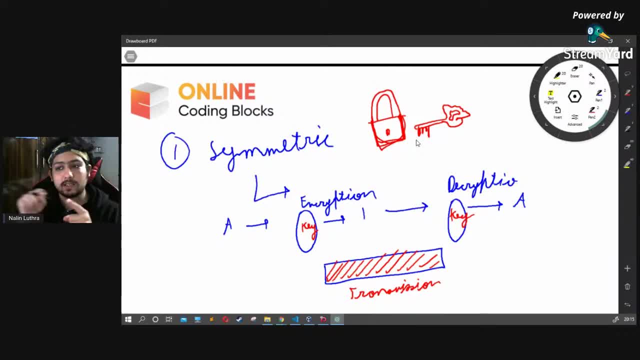 For what To block, For what To block? To block For what For what For block. So I am taking a key which is symmetric And I am using this key to unlock it, So this we will call symmetric cryptography. 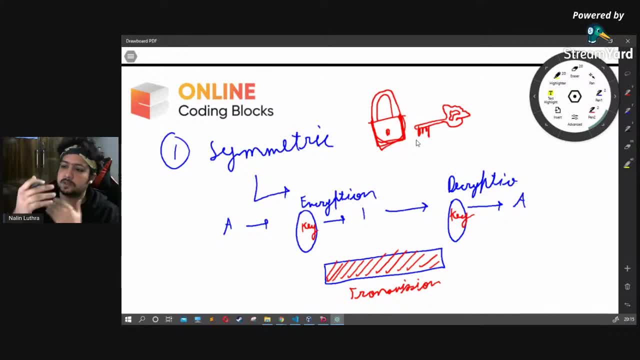 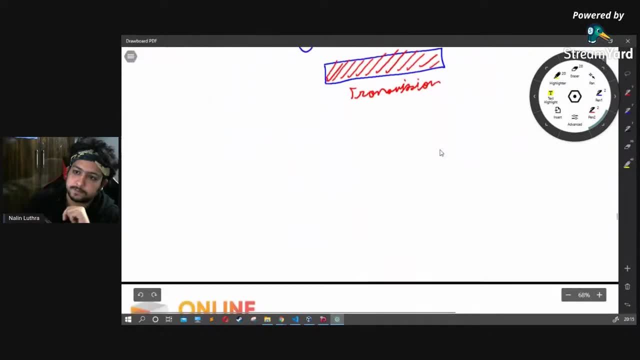 It is quite simple, It is fast and it is used when we want to exchange messages from one place to another. Now we will talk about asymmetric, So let's move forward and talk about asymmetric. Asymmetric cryptography- Okay. So let's move forward and talk about asymmetric. 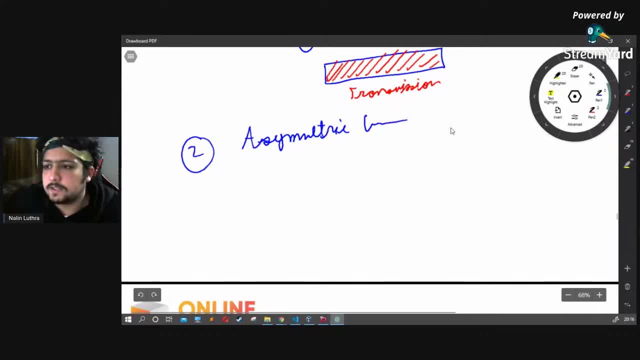 That is the key to block Asymmetric cryptography. Okay, guys, so what is asymmetric cryptography? Wait, wait, be patient. I am telling you. Now we come to asymmetric cryptography. So what exactly is asymmetric cryptography When we use different keys? 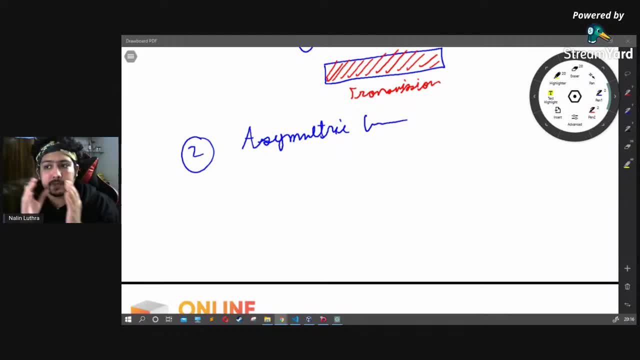 for encryption and different keys for decryption. We call that asymmetric cryptography. What's the matter? Is everything clear? I have a key here which I am calling 1.. And this is my key 2.. I am doing encryption and decryption. My writing is so bad. 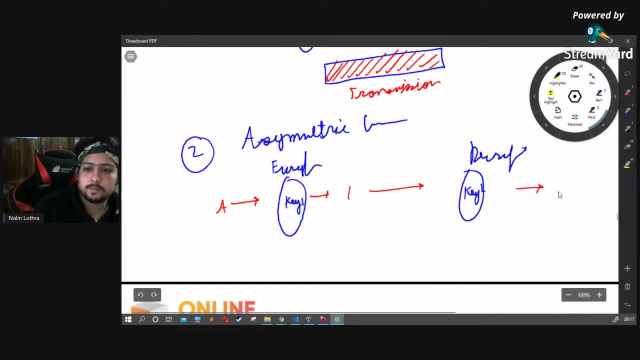 So this is 1.. But in this case, wherever the key I am using, I am encrypting. I can't decrypt it with that key. This is very important to understand If I am using key A. So let's see this. Let's see it with drawing. 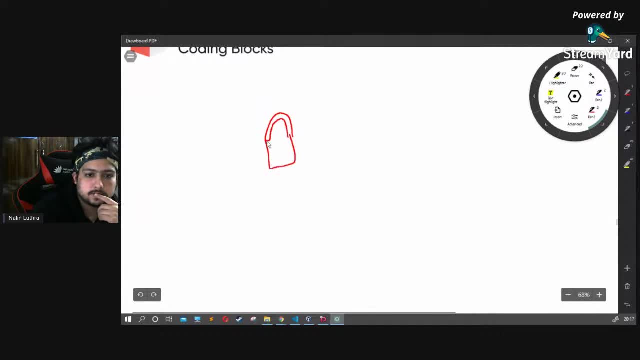 I think drawing is very cool, So this is my drawing. I can become an artist if I draw properly. What do you guys think? I don't know, Maybe I can become an artist someday, Right, I don't know. Okay, So I have key A. 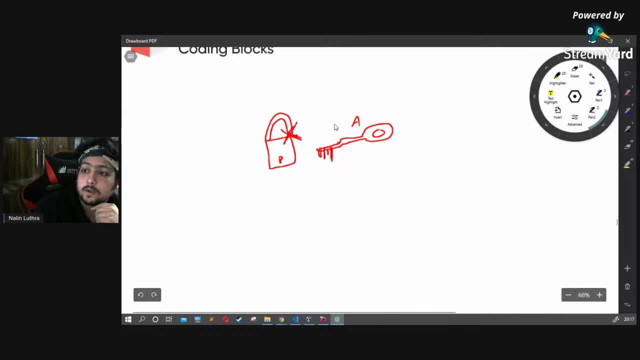 I can lock using this key. It is locked, Okay, But I can't open it using this key, So I am locked. If I want to open with this key, then what will happen? It won't open. For that, I will open it quickly. 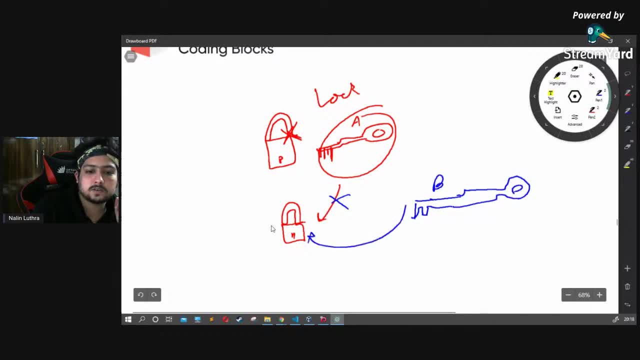 So that it won't be boring B, I will have to use this key to open it. After that, it will open. It will open, Open, Close, Okay, Okay. So this is very important to understand. So the key, I am locking. 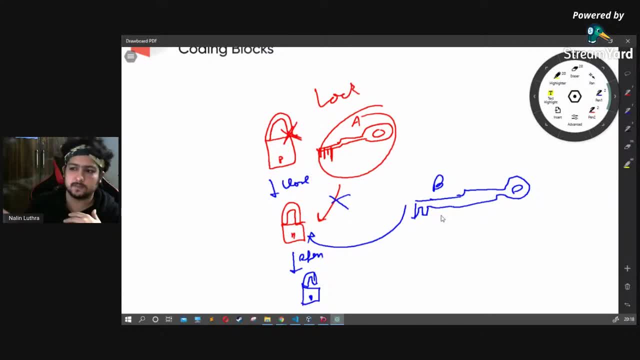 I can't open it with this key, And vice versa, So this is called Asymmetric Cryptography. Cool right, That's how it is. That is where maths come in. This is where maths comes in When we play two keys with one lock. 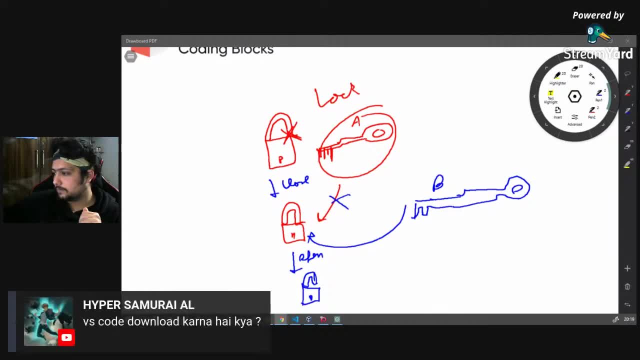 then maths comes in. That's a cool thing, right? No, it's not necessary. I did it so that I can teach coding. So I can write it in VS code Or in Python or any other term, It doesn't matter if you want to write code in Python. 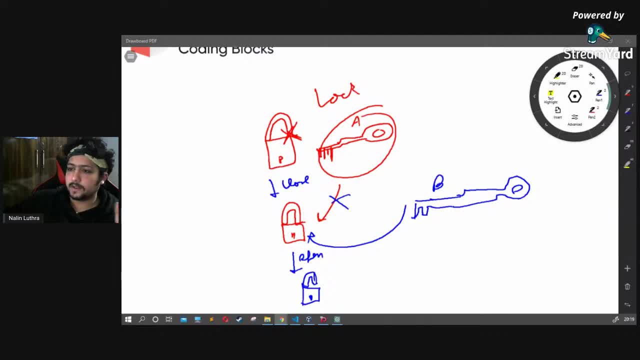 You can write it in Notepad, There is no problem. Okay, Let's move on Now. the most dangerous and my favorite comes hashing. Right Now, we will talk about hashing. Yes, Ujwal, Cryptography is mathematics. 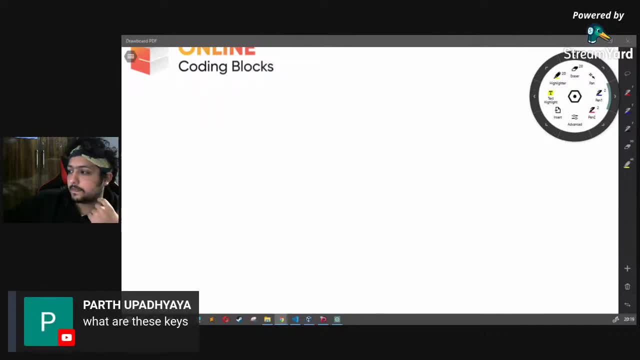 Ujwal Parth, right Parth. So what are these keys? So these keys are basically your codes which are used to unlock it. Like that's how it goes. What should be the right terminology which I should be using for you to understand it? 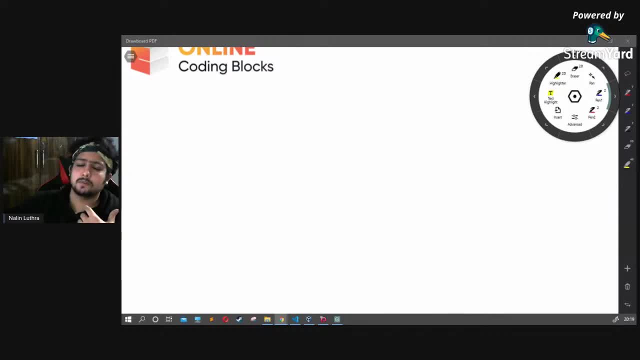 We will, Okay, so think this key just like a lock and key. this is also one key which has certain text which is used to actually decipher it. Yeah, We will talk about that. Give me a minute more on that. I will explain you much better. 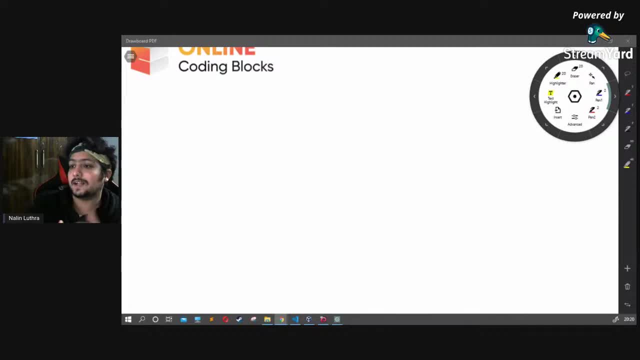 then we will go deeper. Oh, that's cool. Okay, so let's talk about now number third: Hashing. So why is hashing important and why hashing is useful? Salting, I don't know what you are talking about. 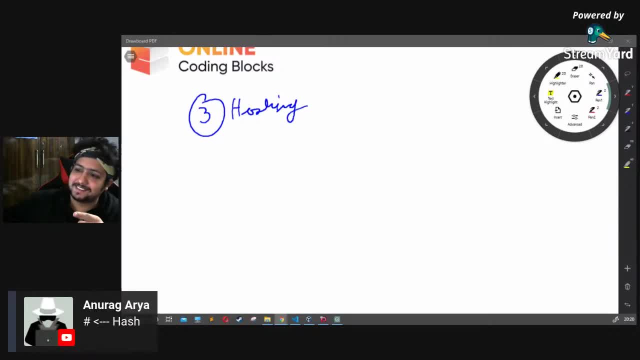 What about salting? I don't know. That's not what hashing is. That's not what hashing is. Okay, I don't know what is salting. I don't know what is salting. Maybe I know. I don't know the terminology. 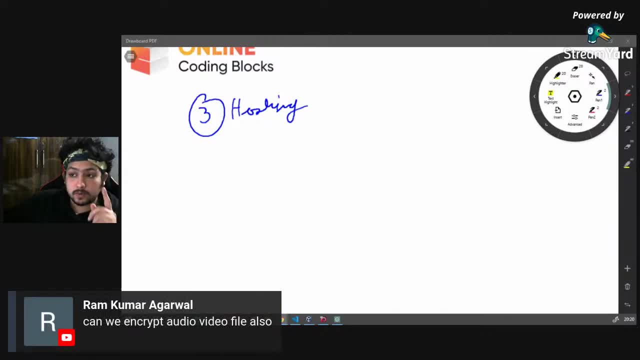 I don't know. Yes, you can and we will do that. Yeah, we will do that. Now let's talk about hashing. Till now, we have seen about cryptography and ciphers. In that case, we will use one key. 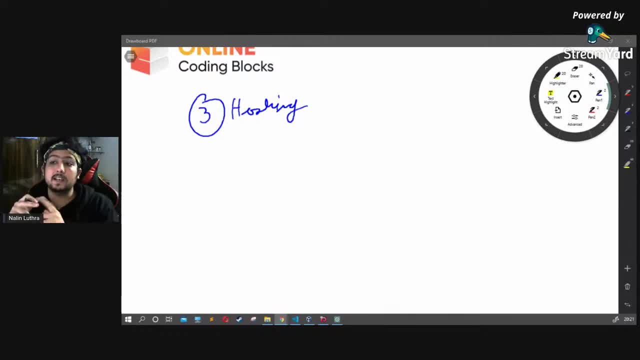 or we will use a function to encrypt something and another function to decrypt something. That's how we are moving forward. In case of hashing, we make something from A to B, but we can never make A from that B. We cannot make B, sorry. we cannot make A back. 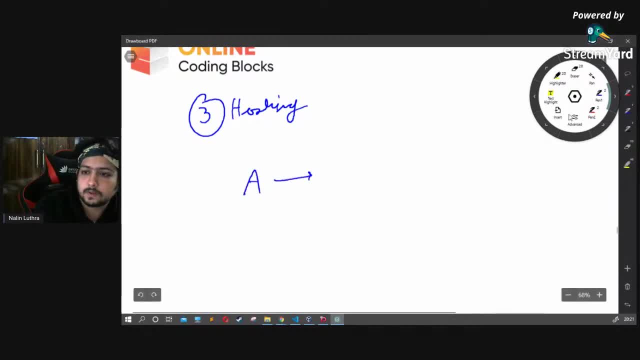 Let's figure it out. We have A, We have this beautiful hash function, Okay, And I get out of it B. right, I can never go back to A from this B. I cannot make A again from B. This is hash. 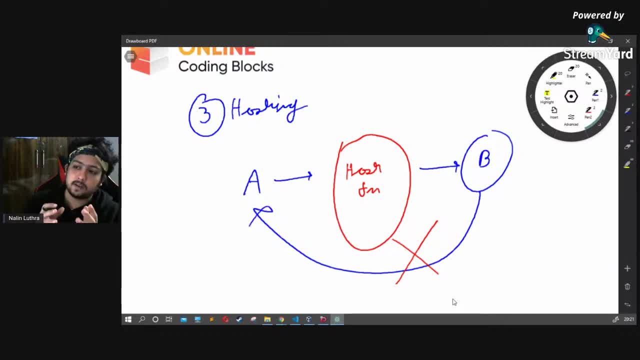 It's always one sided. Symmetric cryptography and asymmetric cryptography are two sided. They have two ways. We have encryption and decryption, But hash functions do not have decryption. It has only and only encryption. Right, Is everything clear? Is this clear to everyone? 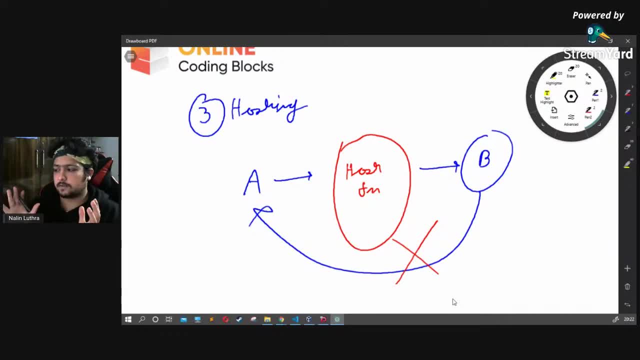 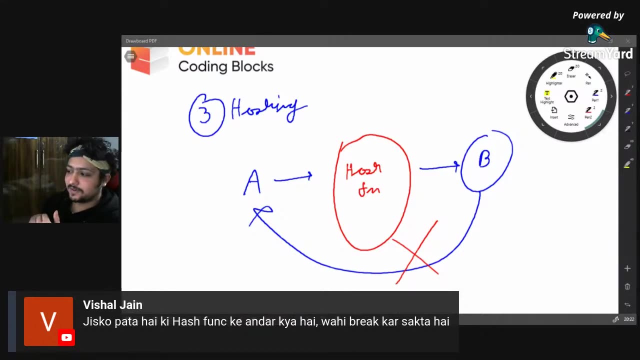 that what is hashing from basic like Right, Okay, Vishal, No, Even if you know what is inside hash function, you cannot break it, And I will give you an example for that. It's a beautiful, simple example, and everyone, those who have done, 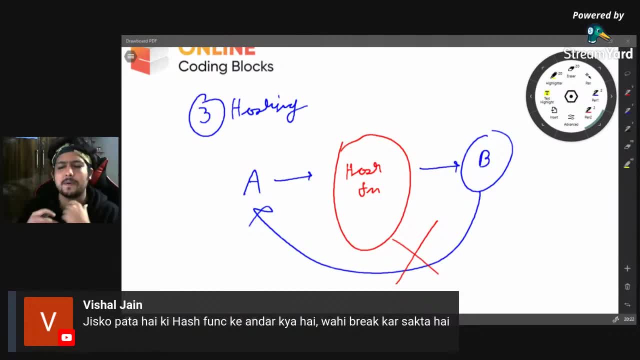 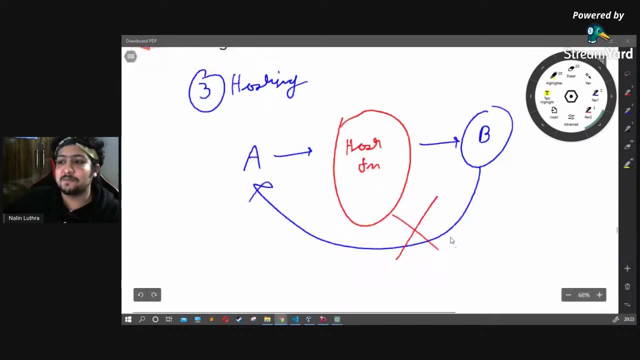 Python has or might have used it once or twice, or maybe n number of times. That's the beautiful thing about it: We don't decrypt it. Yes, I will tell you why we use hashing: because that's an interesting story and an interesting philosophy. 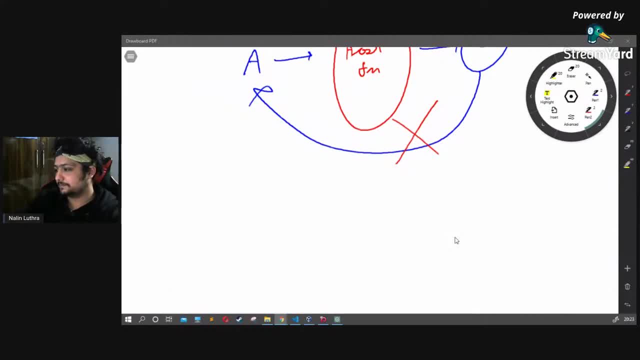 I don't know what should I say? Okay, so That's right, Tanay, That's right, That's right It is used for. Okay, We will give an example for asymmetry, Symmetry and hashing. Don't worry, Today we will give it to everyone. 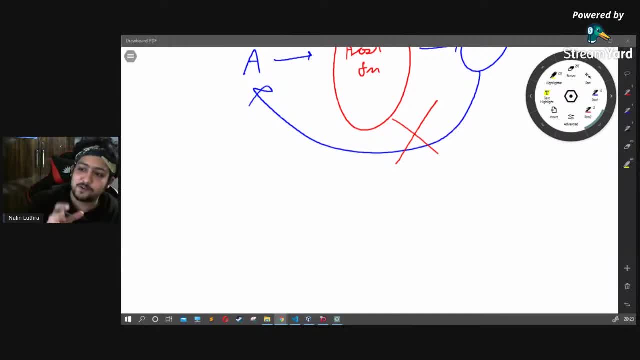 We will give all the examples. Okay, guys, So we will talk about hashing and why it is used. It is very interesting, So this is a story which is not too old. It was 10 years back, So I don't know about the use. 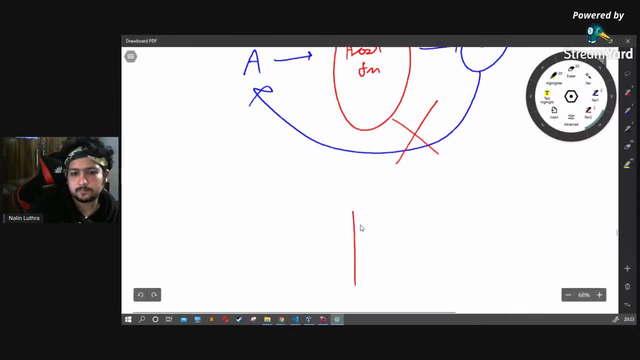 but what happened was there was a very big company. It was a very big company. It had a database. In that database there was an email id and there was a password. Right, Everyone used that. Everyone has a database- Google, YouTube, etc. 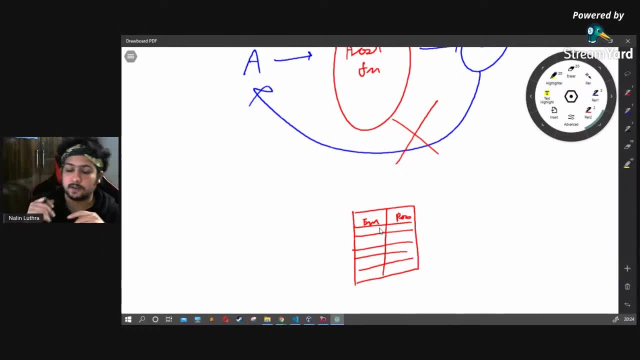 Everyone has email ids as well as passwords, Right, But these passwords are written in simple text format, Meaning ABC, CDF, something, something or something, something. If I encrypt the passwords, then they can be decrypted. What happened? A database of a company got hacked. 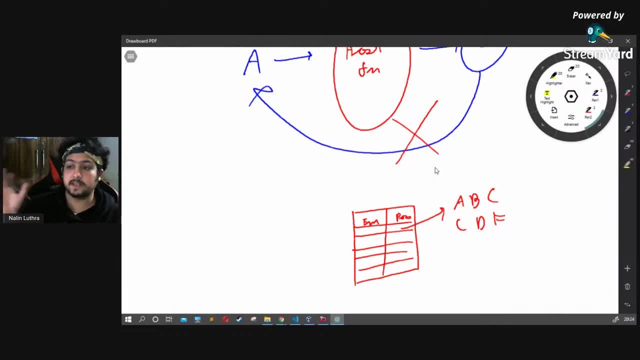 And this was the biggest database hack and like biggest ever. After that, about millions of passwords were found And this is something to understand. This is something to understand a little philosophically: Passwords we normally keep same. For example, if you talk about me, my Gmail. 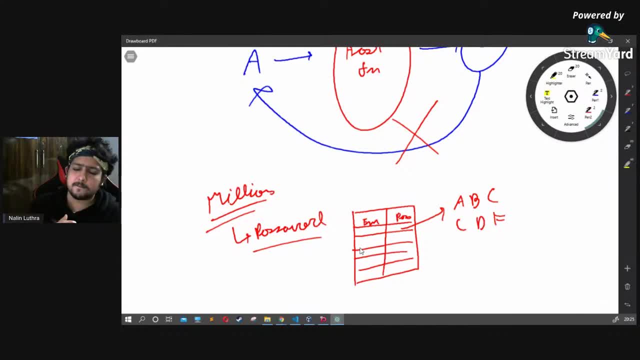 YouTube, Facebook, WhatsApp And all those passwords should not be mentioned. but But whatever, All my passwords are same, So if someone has my one password, then will they get all my passwords Right. So what happens? That company's database got hacked And the reasoning behind it. 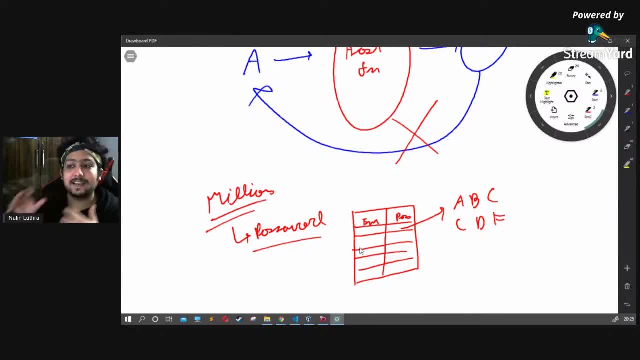 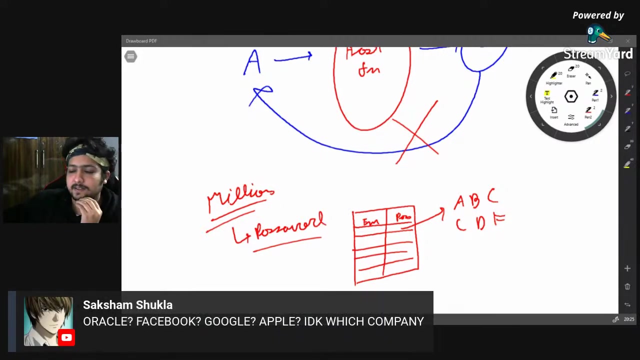 is that all the passwords got leaked. These got leaked. I forgot the name of that company. I will let you know, guys. I will definitely let you know guys. Right, So one gone, all are gone, Right, No, guys, itni badi company nahi thi Chote company thi It. 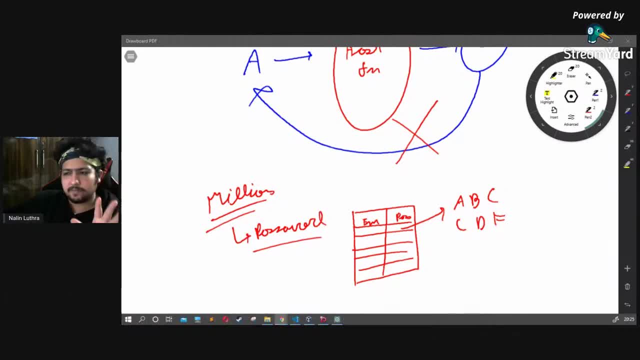 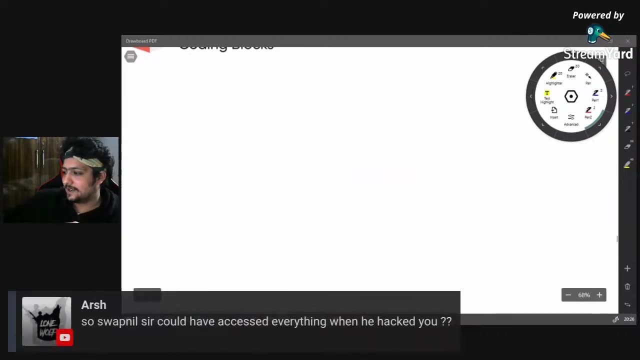 was a decently big company. I forgot the name. Give me a day's time I will let you know. Usko bhulte hai. Let's forget about the company. Let's move forward and understand how important hashing is now. No, it's not Cambridge Analytica, Not really. I am much smarter than that I have. 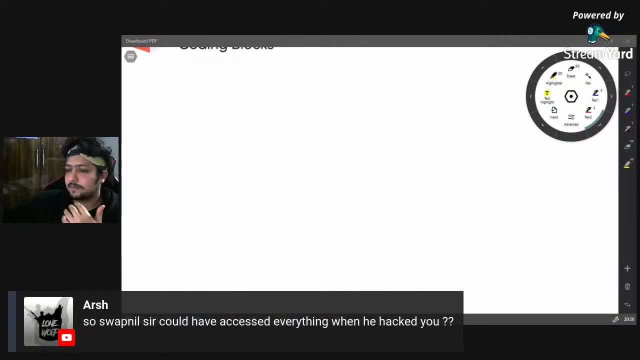 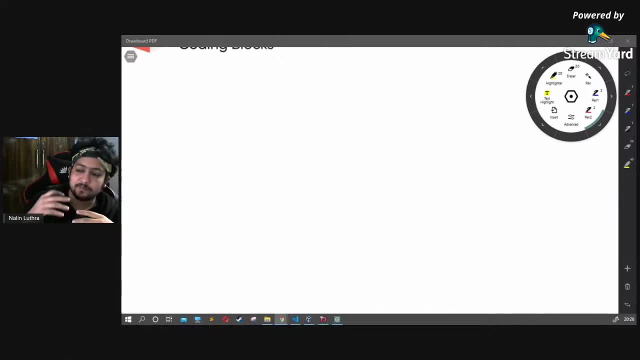 written some scripts which change password instantly. whenever I feel like something is going wrong, Password gets changed instantly, Like bam done over. So coming back to the game, So what happened was siren password leak over. So that's where hashing is important. So what we do is, for example, mera password hai null in 1,, 2,, 3, 4.. 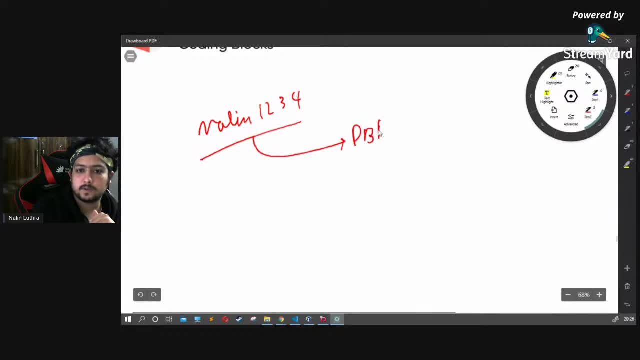 Right, Agar main database ke andar isko direct store kar dunga, Okay To ye galt hai Wrong way. Okay, Us case, mai kya karta ho? Main null in 1,, 2,, 3,, 4 ko convert kar jata ho, Ek hash function. 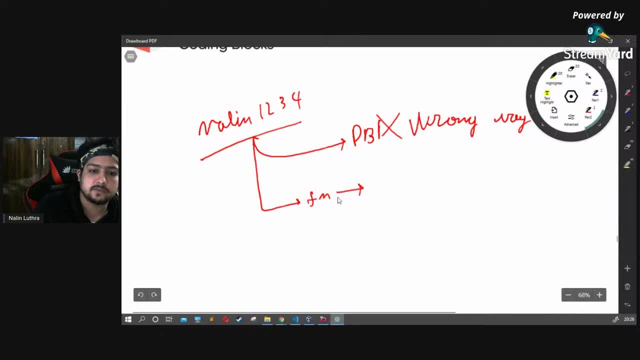 kar jate ho. Okay, To yaha pe function jayega Hash function Aur mere paas output aayega Kuch random likha hai. That's completely how it goes. Ye jo, hash function, mere paas aaya. 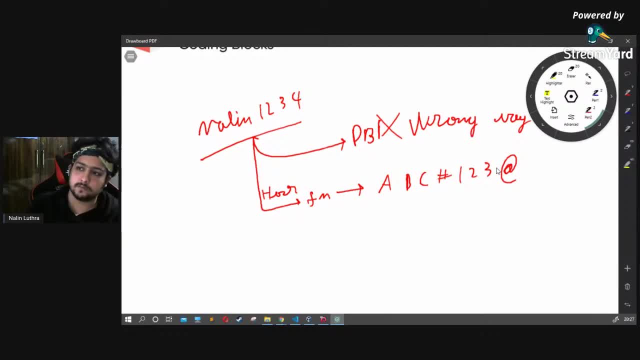 This hash function will always be same whenever I write null in 1,, 2,, 3,, 4.. Matlab hash function kabhi bhi change nahi hota. Kaise matlab, Agar main usme bol raha hu, ki main null in dal raha? 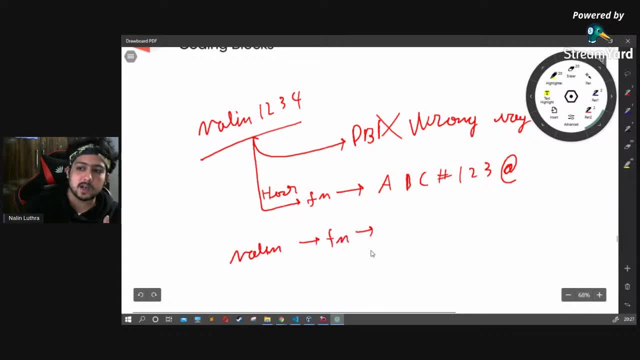 ho Aur usko mai function se pass kar raha ho To mere paas humesha output kya aayega: 1, 2,, 3, 4, 5.. 1,, 2,, 3,, 4, 5. Ye. 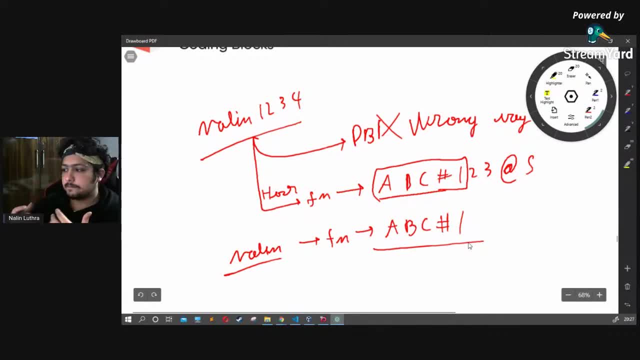 So ab jab bhi mai dalunga, ye output aayega. So companies ne kya karna start kara. they started storing passwords in hash format. Hash format mein save karna start kara, Agar database hack bhi hogaya, Agar saari database. 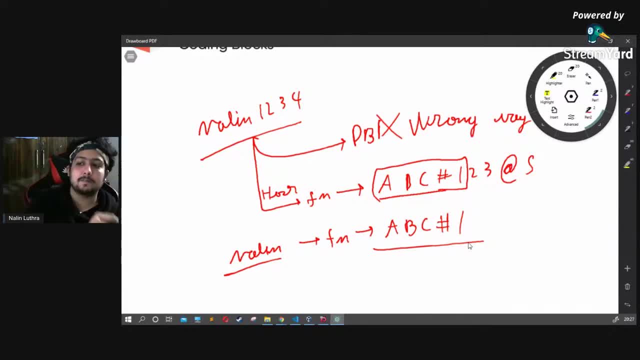 hack bhi hogaye, they cannot ever find out the real password. Right Kyunki system hash match karta hai, not the password itself. To jo urse ek hash generate hoga, it will match that hash and not the password. Kya ye cheez sab ho clear hui, Yes or no, Right Kya ye? 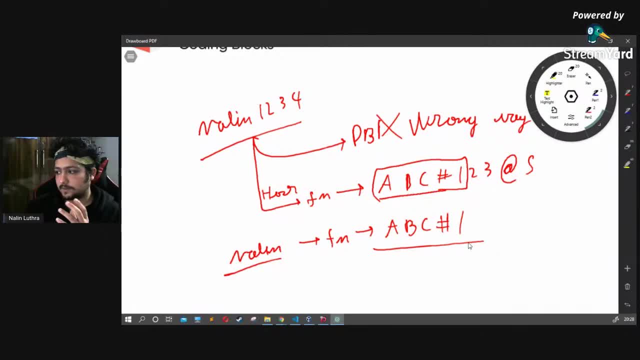 cheez sab ho clear hogayi hai. Ye hash ka use kaha pe hai? It is used to actually store passwords. So we can compare those hash values to find the real output, Right? I don't know Once more. Okay, Vishal. 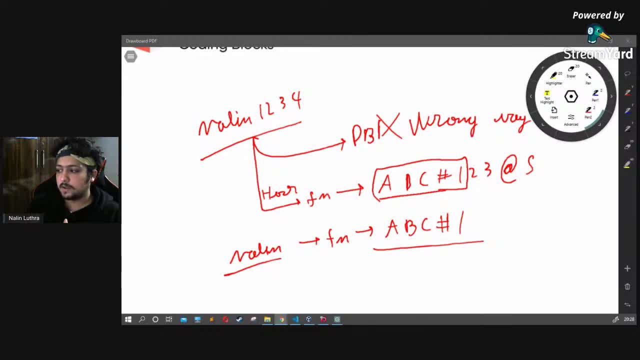 It's simple: We never store passwords, We never store anything. So So I'm not sure about it. Again, I'm saying I'm not sure. It's something called u-hagged or something I don't know, U-password list, If you just google something as password. 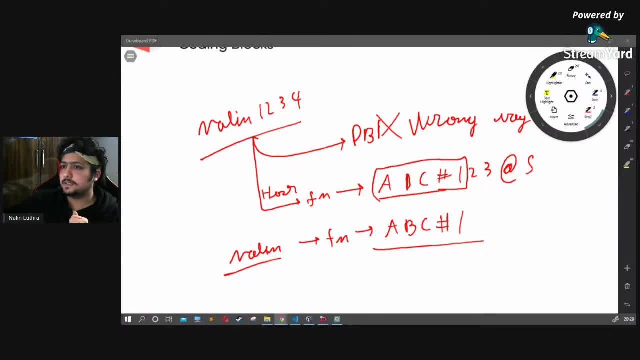 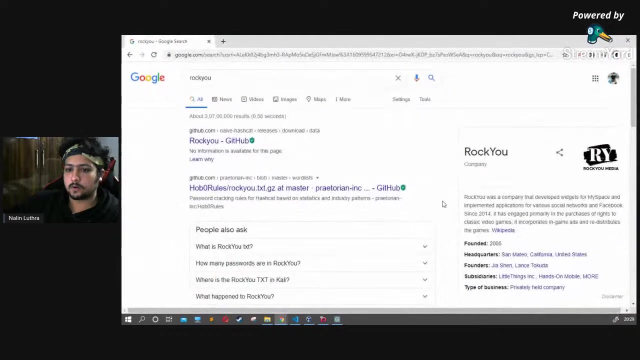 list kind of thing. you will find it. Let me see if I can find it for you guys. Rock you- Yeah, It is called rock you. That's how it is. It is called rock you, That's the name. So rock you was a company which developed widgets and everything. So this was a company which. 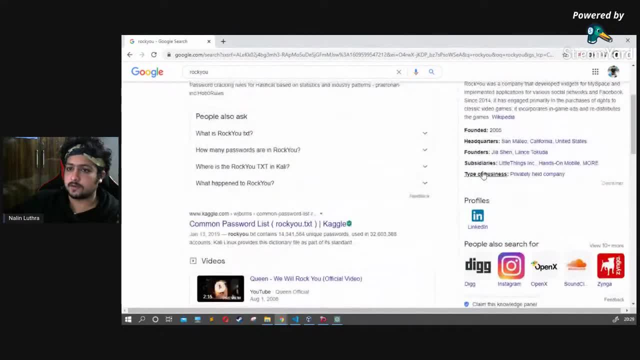 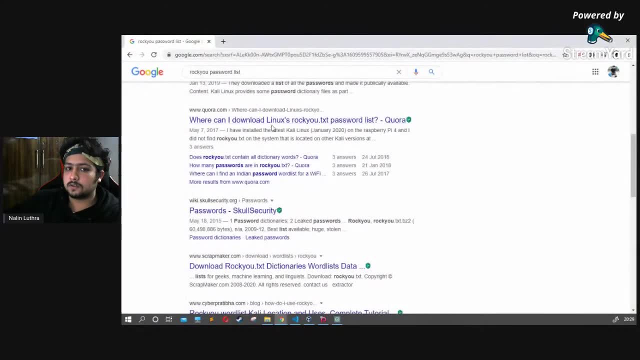 ran bad, I don't know. Yeah, this was the company which ran bad, So it's called rock you. And now we say rock you password list, So rock your password is basically list of all the common passwords which people use, Like doj rho. Heavenly bha have n have garb har awesome past right. Like 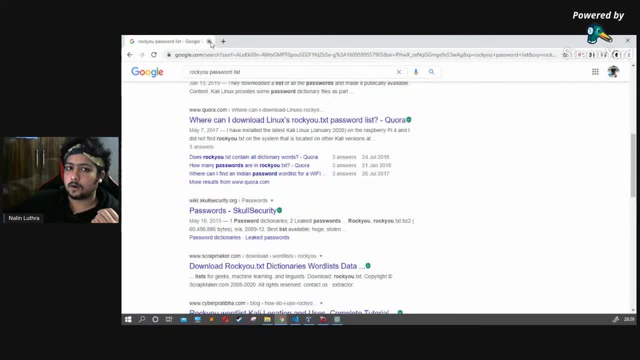 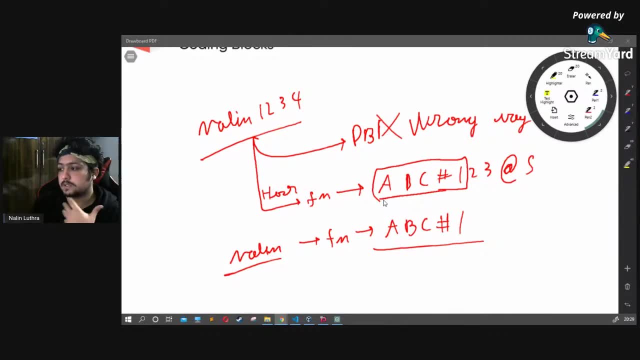 like pass one, two, three, four and stuff like that. so it's called rock you okay, so that's, that's how it goes. so now, then they change everything, and now we actually can't access the password, so you only get hash. so the most beautiful thing is, even if even- okay, actually all these passwords are hash, are converted, 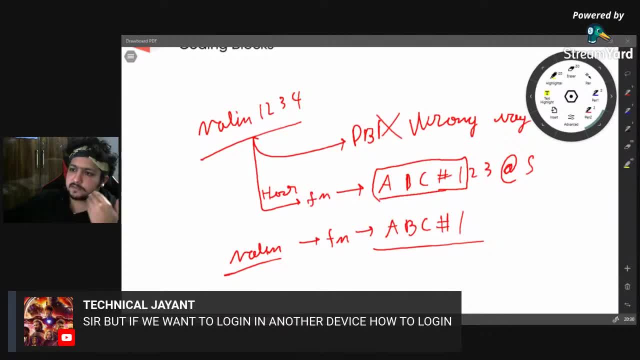 and stored in the back-end itself, not in the front-end, means device to device it won't vary, it will be constant, because everything is happening at the back. we just send the data there. it changes with magic and it gets stored. yeah, don't, don't, don't do that guys. 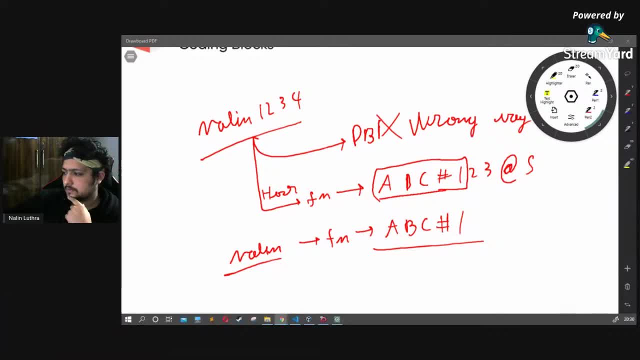 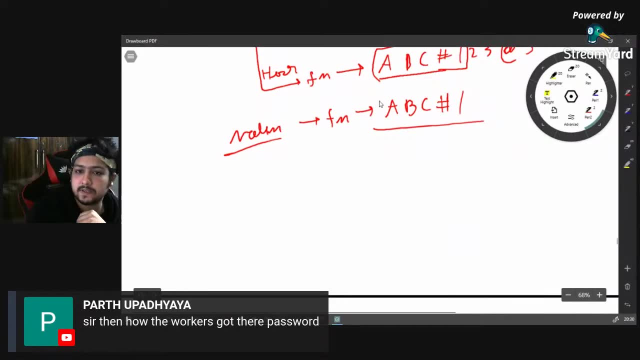 don't. don't do that, okay, so you don't need passwords in that case. now we need hash. now what I have to do is I have to store what I have stored in the database, right? so whenever I have to do it, I have to do it in the back-end itself, not in the front-end. 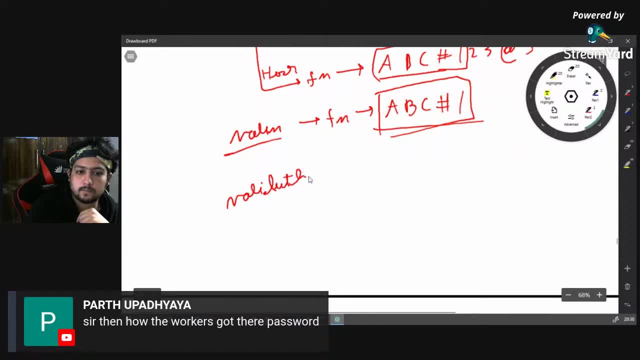 I will write nullin dot luthrat, the rate gmail dot com. okay, in that case, what will happen with me? I have gmail dot com. with my this id, what will I send? my password, which is nullin, one, two, three, four, right, this whole set will go. this id will remain the same as it was right. id will remain the same, but. 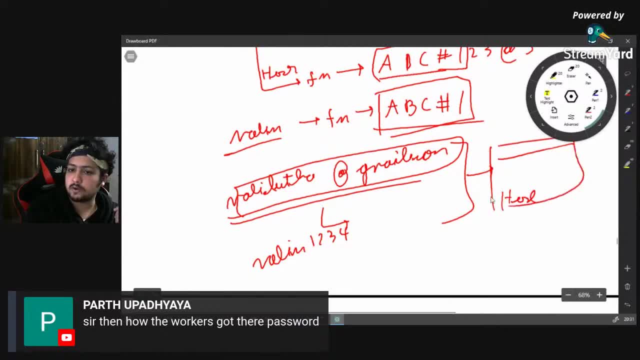 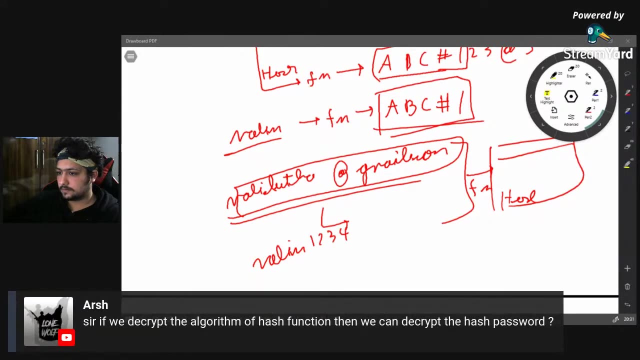 my password will change in the hash and that hash will be stored and whenever I pass, it will always be the same hash. right, it will always be the same because before we match, let's convert it again. that's simple right. no, you cannot. that's what I'm saying. that's the beauty of it. 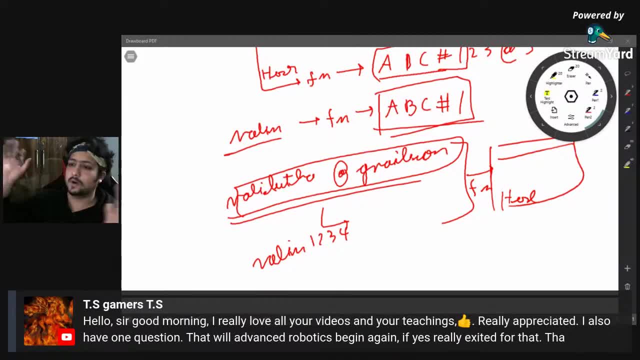 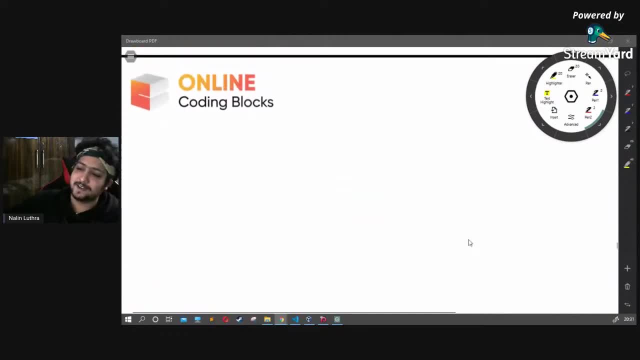 yes, we will do advanced robotics. I promise you on that. after this, we will do advanced robotics. that's one and for all. I got you. give you the answer. who gave the answer? Nalan gave the answer. We will do advance robotics moving forward. now let's see why it's not possible to. 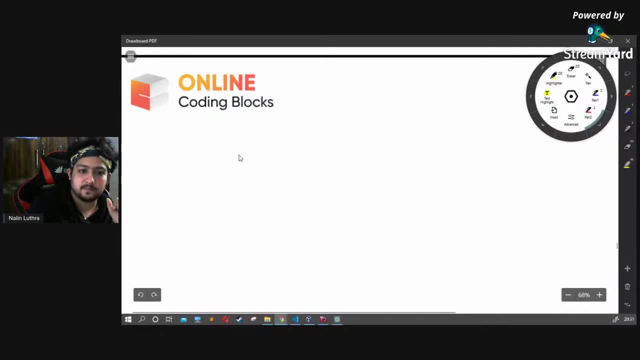 reverse the hash altogether. 7 include this output. Wow, how does 7 compute mod mode 4? No, Now 19 ín this output. NO, fast, fast, fast, fast fast it's got off. seven more for God would get over 19. what for God would get one. three more for God would get one. first, three, right three. 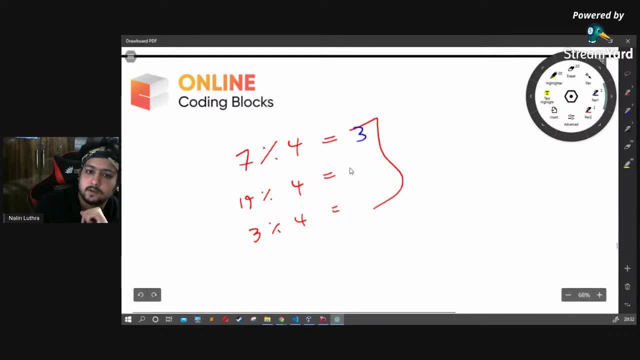 everyone got answer: it's three, three, three, right wrong, Chaitanya, everyone output goes for three because dots are what? these, what functions are for right? don't don't spam, guys, don't spam, please don't spam, all right, everyone is saying three, three is the answer. this is my hash function, the most basic hash. 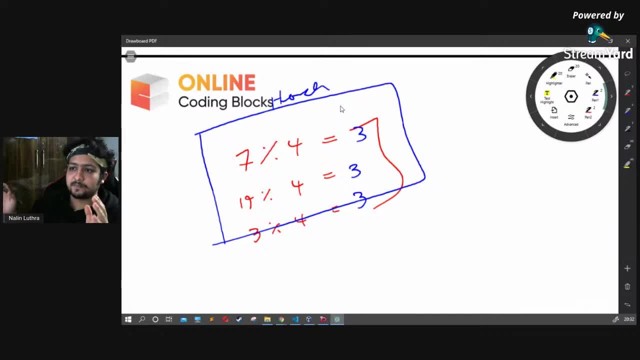 function most basic, right, this is the most basic hash function. so what is hash function mod for? this is a function. now, even if I give you the hash function, you cannot reverse this. so you have three, three and three. now tell me how this three, three, three becomes seven, nineteen and three. it simply 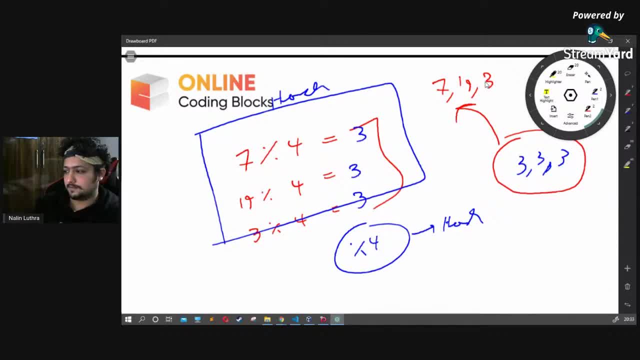 cannot. you can never predict it. right that this is what you get exactly. that's my point. you can't tell and that's the story behind it, guys. okay, so that's how it goes. this is what hash means. so does everyone understand? what is the use of hash? how has is beneficial, why we use hash and why not? 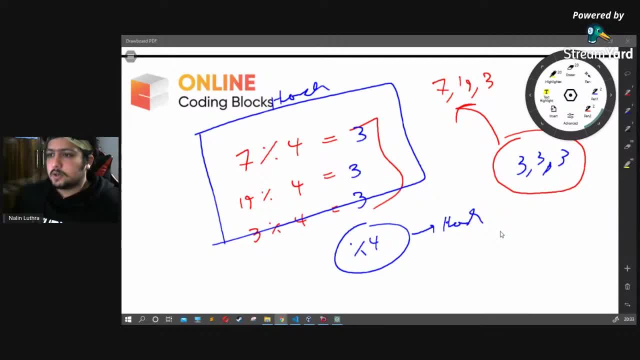 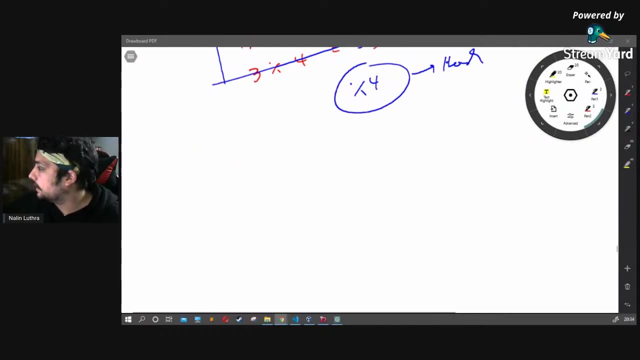 right, who should we start some coding now? which port? here's a? here's a unique user code. okay, so so say: fellow code, home time. yeah, oh, she doesn't have a cousin. that's an interesting side, so we will start with see the side. what so they? 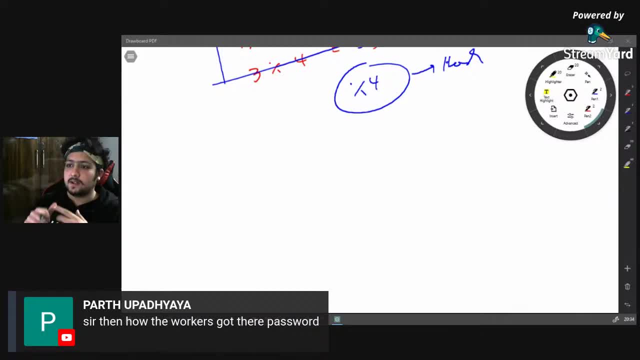 don't know what. neither Gmail, no Google can read your passwords. no one can here. oh, chetan, you got late. that's odd. so we talk about hash, asymmetric and symmetric cryptography. clear- it should be clear, not clear. that's weird. okay, white white. okay, coordinate, symmetric- we'll talk about that. 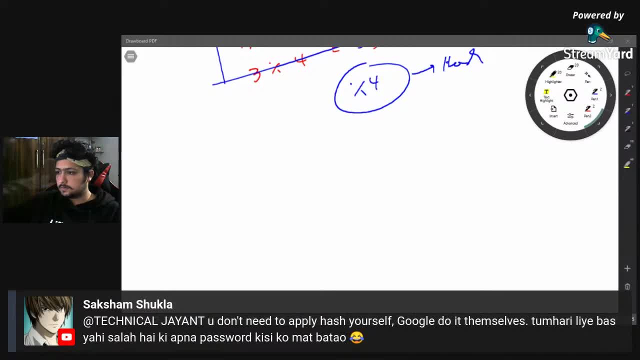 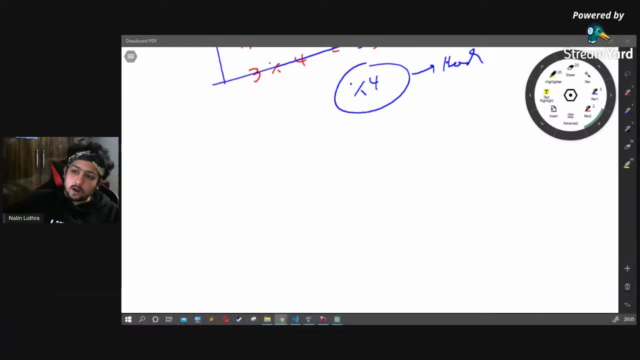 right. thank you, section. so much for that. that's right. so now we will talk about caesar cycle. it is never decoded. it is never decoded. that's what i'm saying. it gets encrypted and saved in encrypted format, hash format. okay, so we will check hash. okay, it is never decoded. it is never decoded. it is never decoded. that's know. 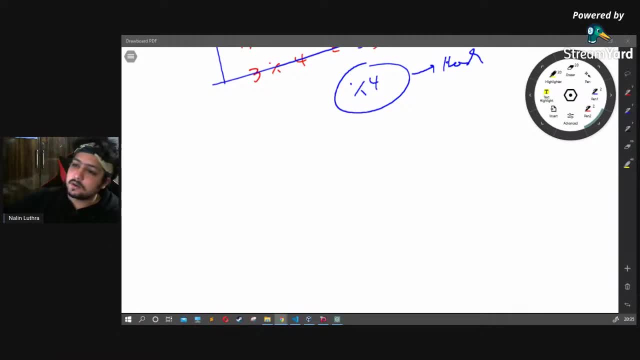 it's not time to split it. we are talking about hash over here at the start of the second chapter we will talk about it is never decoded. it is never decoded. that is why we are talking about hash. ok, so now in this section we will talk about a very important issue. 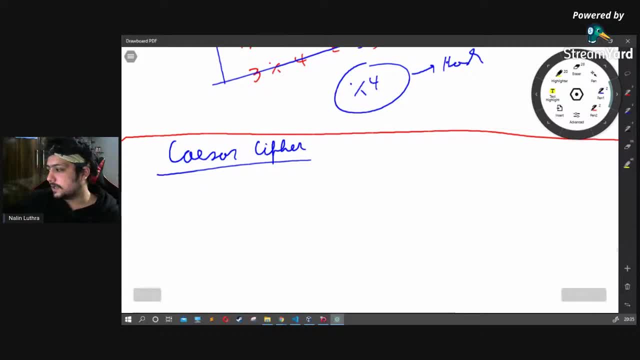 and let's first talk about the next section, the third step, are thinking the cipher is based on julian caesar. uh, that's not true. okay, so this cipher is not based on julian caesar. this is called caesar cipher, right? so if a word will always be same, 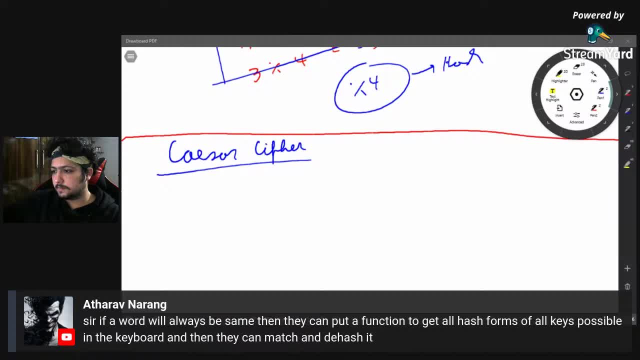 they can put a function to get all the forms of all these possible in the keyboard and then you can imagine no earth. well, because this is the most simple way to hash it. but these days hashing comes in extremely complicated mathematical formulas which cannot be just stored like that. okay, it is. 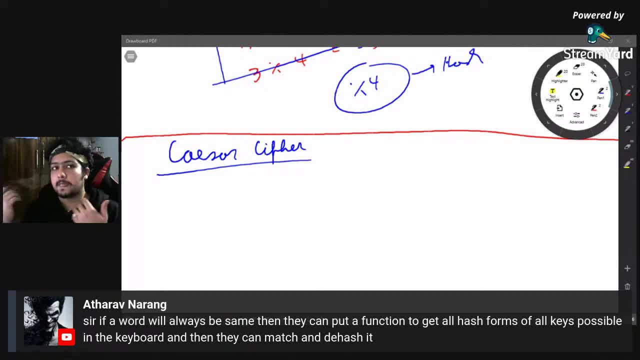 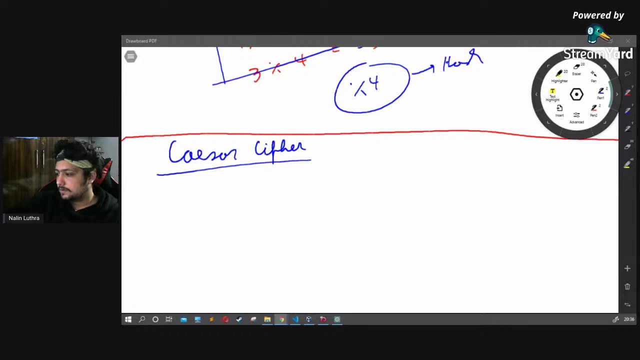 like billion and billion of outputs, with billions of billions raised to power, billions- i don't know, give your biggest number you can think of- of inputs. so you just cannot. okay, okay, guys. so, uh, i think should we move forward now? yeah, good enough, so let's move forward. 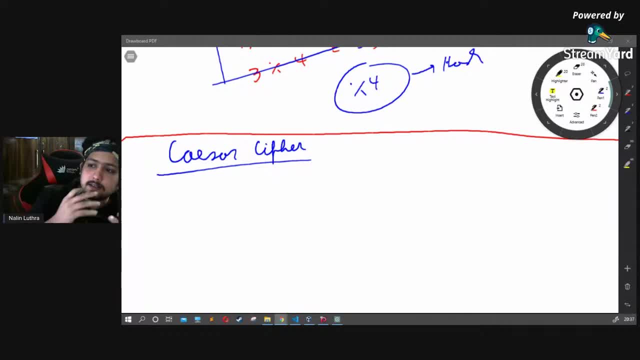 cool. so now let's talk about caesar cipher. so this cipher, uh, is not, i don't know. is it based on julian caesar or not? i don't know about this. some people ask me about this cipher. is based on julian caesar? i don't know. it's a story in your english books, i guess. i don't know. so, okay, so 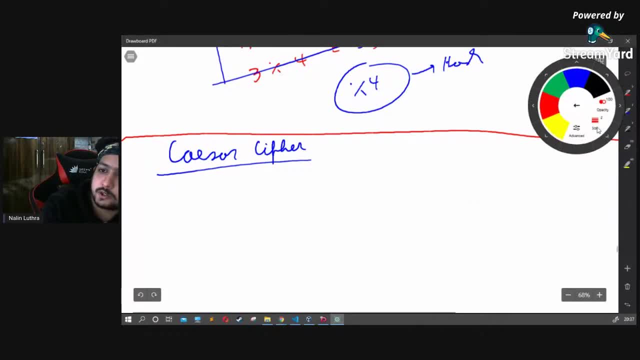 let's move forward now. so cipher may have julian. let's get green now. i've got both the colors, okay, so see the cipher. so how exactly does csr works? what is it csi for? why we need csi for? and blah, blah, blah. so we don't actually need csi for, but it's a basics. 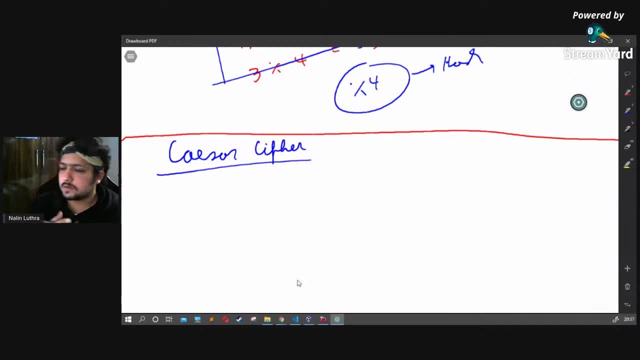 of cryptography. so we'll talk about csi first. so what exactly does is basically it shifts all the value by n, number of alphabets. let's just think like this: so if i got a, b, c, d, e, f, cool, so you say a, e, f, g, h, i, j, k, l, m and let's just do this. okay, let's just do this a little bit. 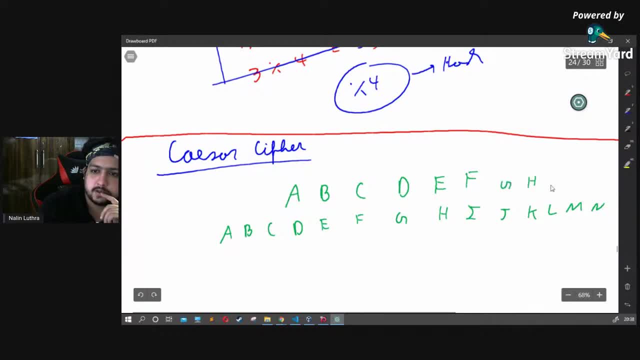 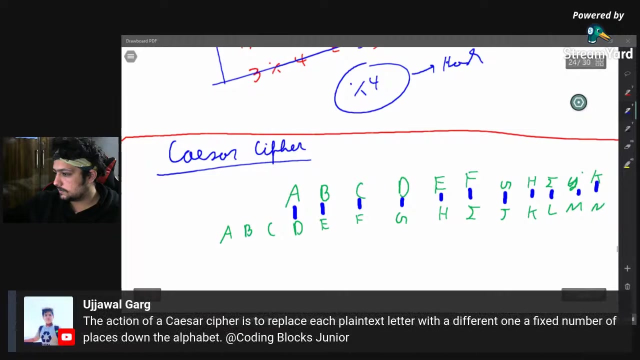 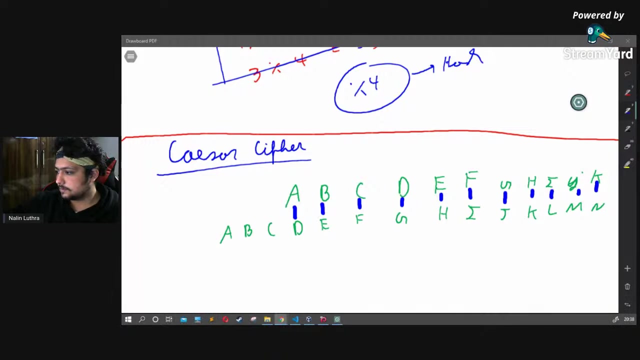 yeah, uh, g, h, i, j, we have j, we have k. cool, okay, so this is linked to this. that's how it's going right. let's try. thanks, okay, good, so ruji pandit just updated us that this cipher is based on julian caesar- cool. 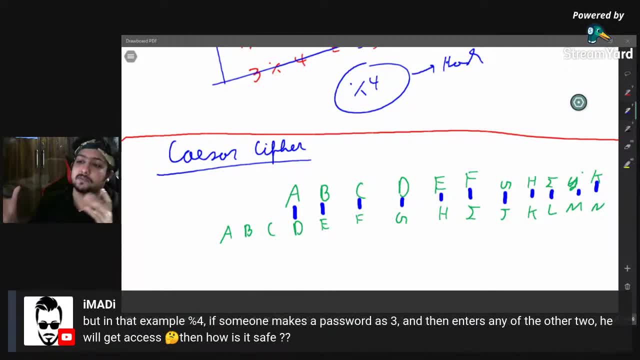 okay, i'm maddie, it's it. this is the most basic hash function. this is not used by google or facebook or youtube or anyone around the world like this is the most basic. just to actually explain to you how these hash function mathematically works. 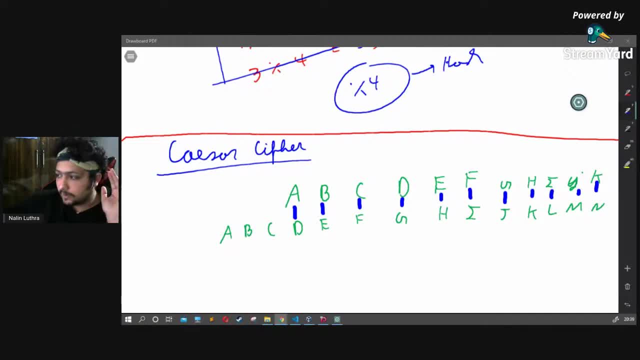 this is not what we use. forget it, we don't use it. it's just for the explanation. okay, it's way too much complicated from that point. all right now, moving forward. uh, fun fact. uh, we use, we use more prime numbers for crypto. we'll talk about that in the next class. okay, guys. so this is called caesar. 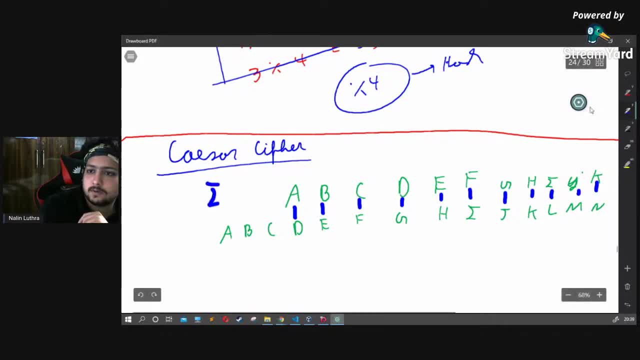 cipher. okay, so this is my input. i don't know why it's so big man, i should just erase this one. okay, so this will be my input and this would be my output. cool, cool, i'm cool, like, done, done. okay, so let's give me quick answer as fast as you can. so in this case, value of n is three. 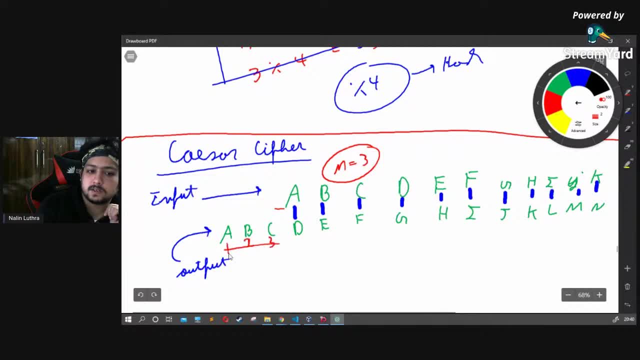 because the rotation is by one, two and three, right, so three values are rotated. quickly, answer me what will be the output of b, c, e, f, h k. quick, quick, quick. what will be the output of d, c, f, f, h, k? if i input this, what will i get as output? if i say a, i will get d, b, c, f, d, g, e, h, f, i, g, j. 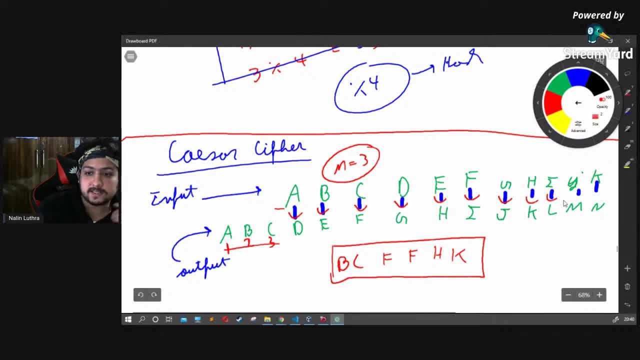 okay, uh, okay, okay. someone is saying ifkin. uh, we'll check about that, if you can have it. i don't know if it's right or wrong, i don't know, i'll check. if many people are saying ifkin, let's hope if karen is right. 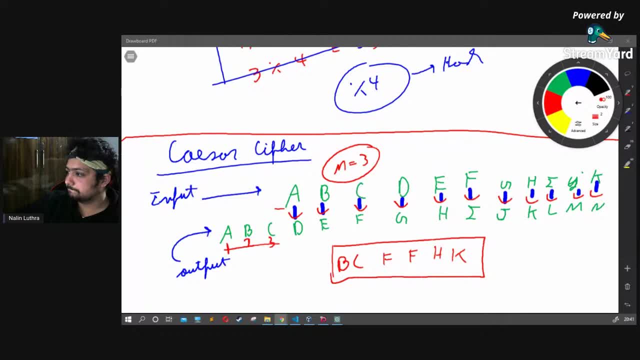 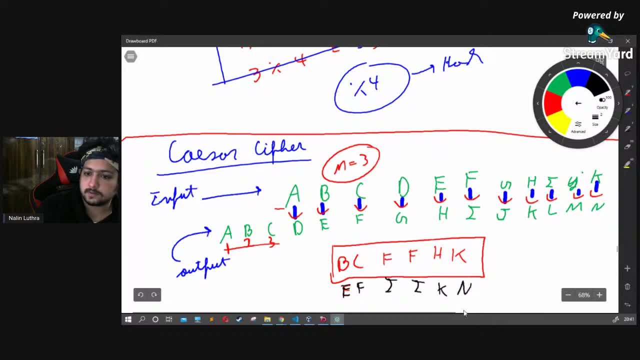 similar camera case in right. so what did i say if kid, if it's good, right, cool, got it, ifkin, cool, yeah, ifkin's right answer. so this is what we call it: a caesar cipher, right? i don't know, man, it doesn't matter if king hiking it doesn't matter what it doesn't, it's not even a. 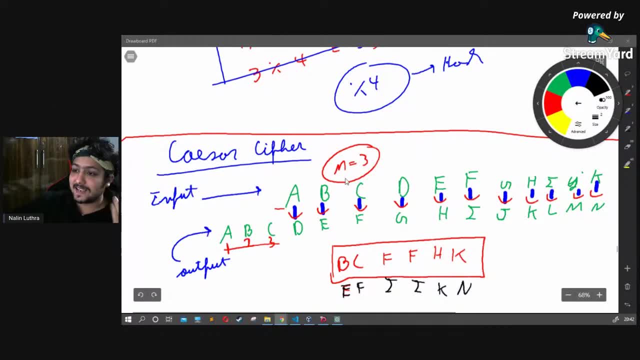 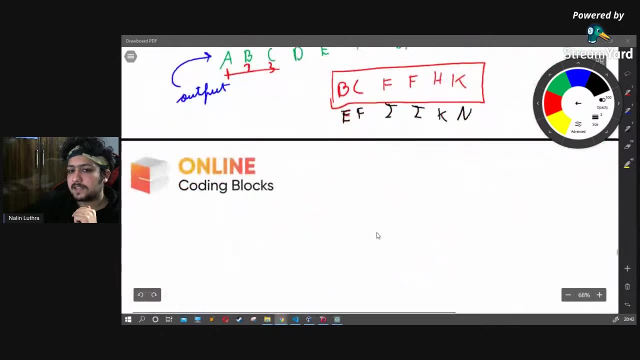 word itself. okay, so what? i'm trying to explain it to you. the value is: n is equal to 3 over here. uh, it is called a caesar cipher. that's all right. so let's start the program to write a caesar cipher. now what you guys have to. 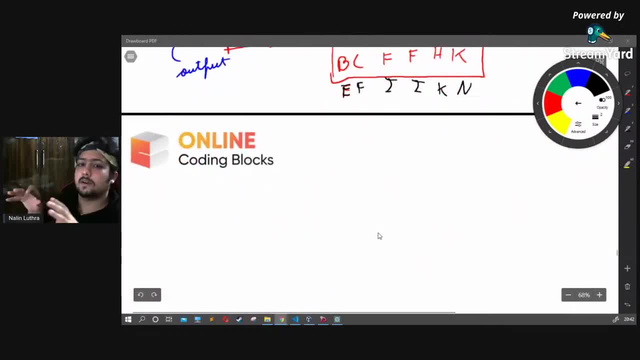 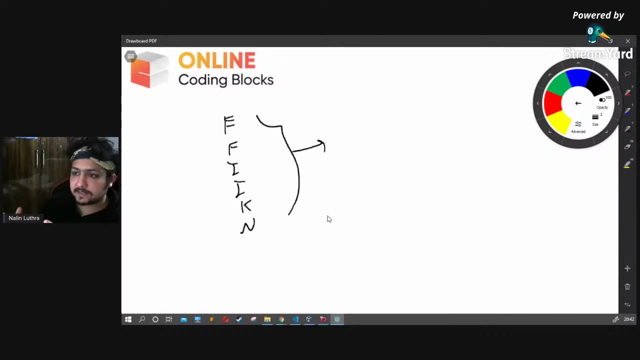 figure it out is. i will tell it to you, but while you're writing code you have to think about it. if i give you e, f, i, i, k, n, right? can you tell me what will be the output of this using caesar cipher, if you don't know the value of n? 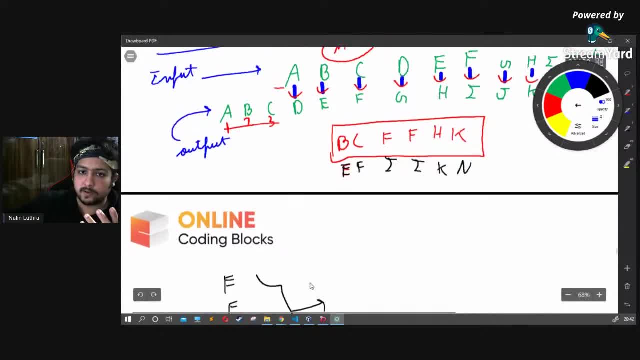 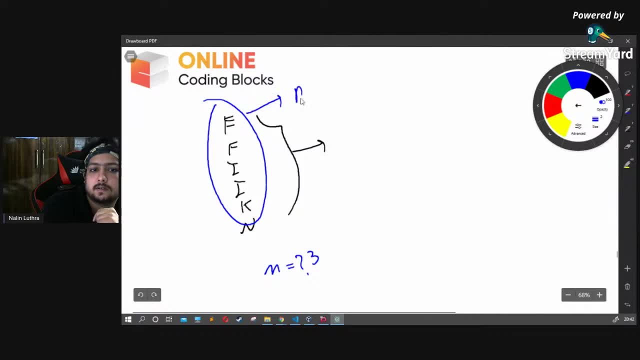 you don't know n, right? you know what n, because i've told you that n is equal to 3.. so if i say n is equal to 3, can you decrypt it? yes, please write a function to decrypt it right. first, we'll start to encrypt it and we will see. 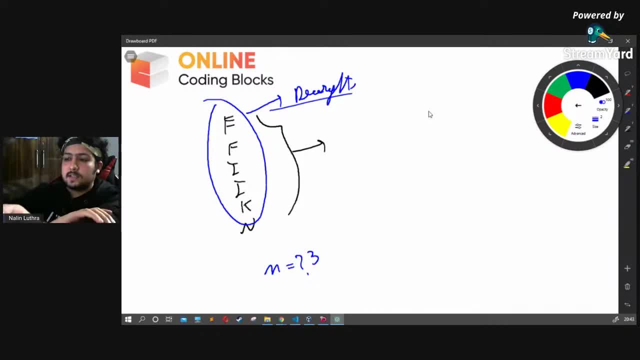 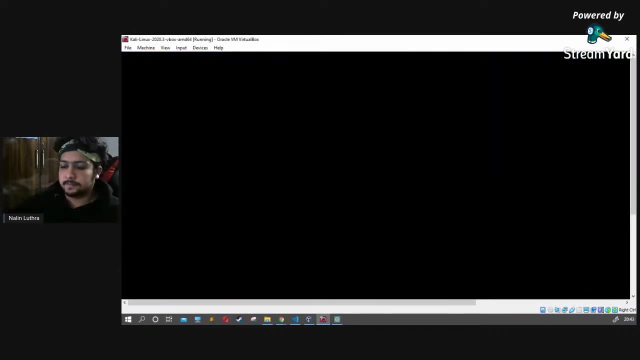 if we've got time to decrypt it as well, to get right. so let's raise our jackets or i don't know like sweatshirts you go wearing, prepare your hoodie and open your variable code so we'll code in kali just to make it work. it feel like it's not really hacking, is just a simple. okay, my, my color is not. 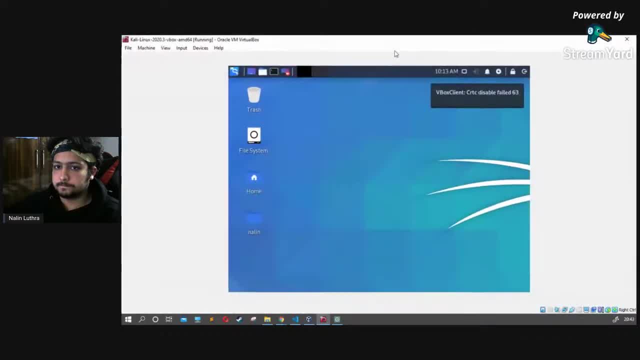 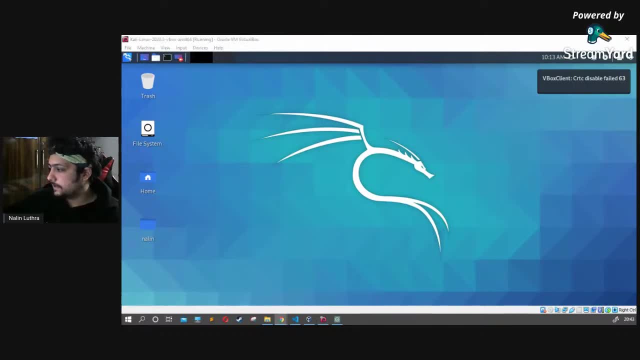 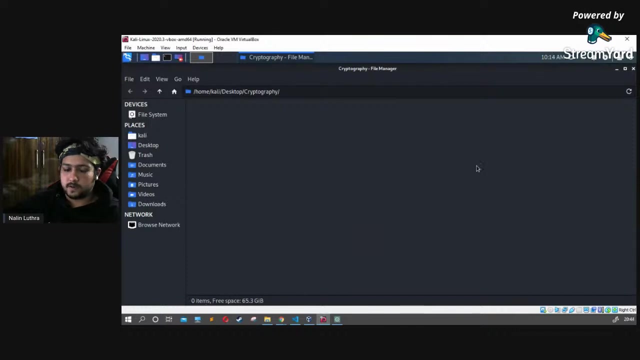 working. now this is weird. it's supposed to be working. that's loaded now. cool, okay, let's start our first Caesar cipher program of what I don't know. okay, so let's make a folder, let's get into it, open it. let's over here, come on terminal. 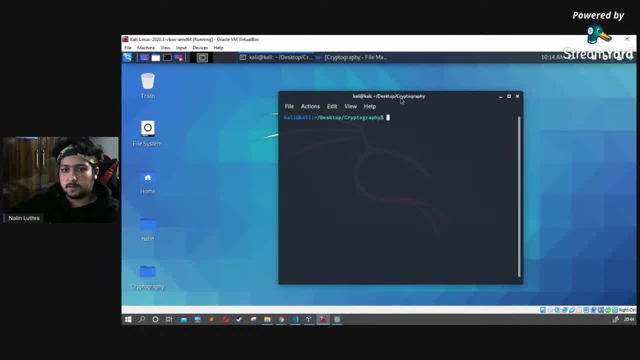 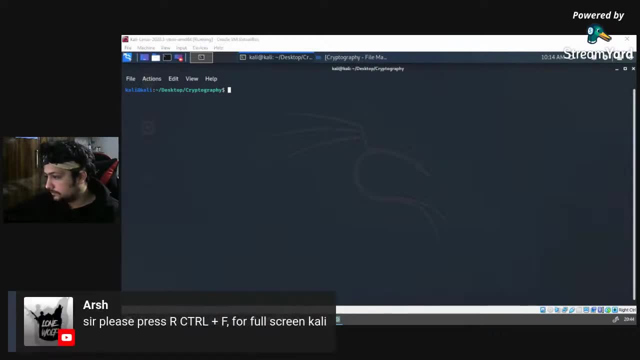 get me what he got. so terminal is here. I will use nano to actually program it if you want, sure, hey, someone is saying you'll make a full screen control if it's not working on tight control per se for full screen. Kali, it's doing it. it's not working, so I 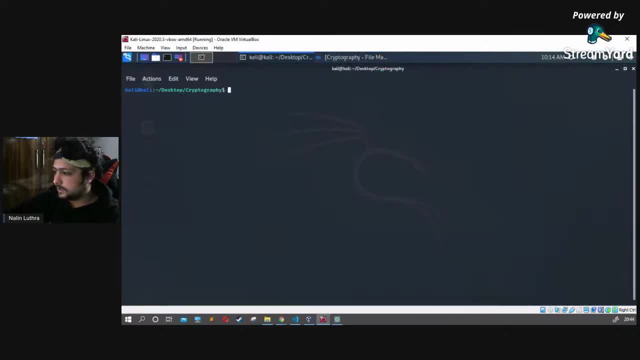 don't know, okay, so let's start coding. guys, let's get up dirty. oh yeah, you can put in whatever language you want which will logic, it's same. I've told you the logic guys, logic, it's same. do whatever you want, okay, okay, okay, okay, I will start nano. you can do wherever you want to do in programming, it doesn't. 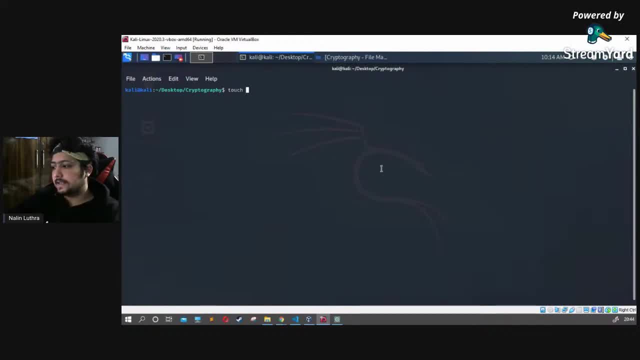 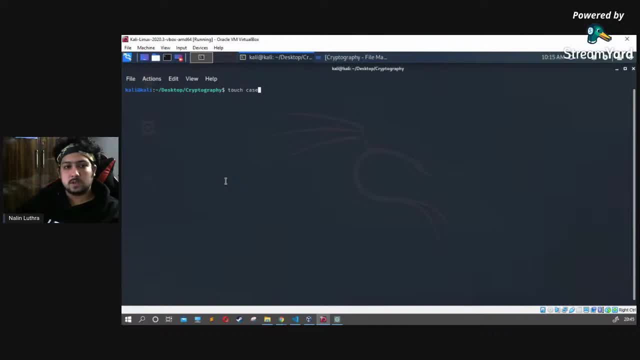 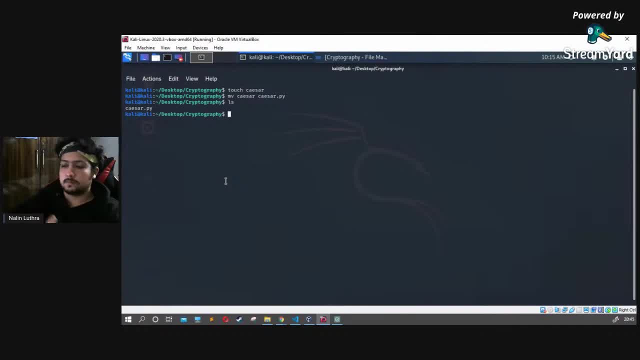 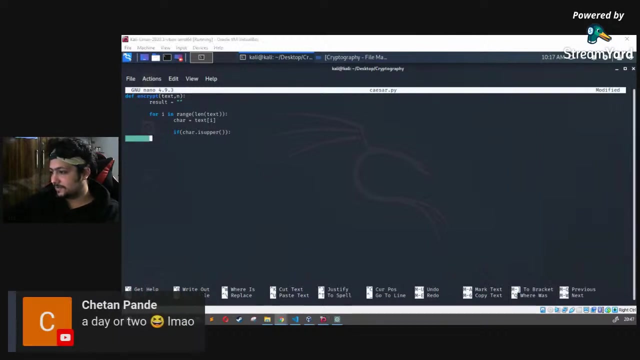 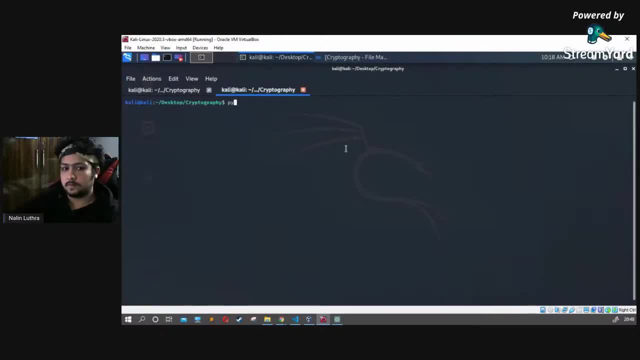 Okay, I will tell you what is ORD, What I will do right now: Python, Right? so if I say ORD N, Well, let's go with 1 for that one. It's not working. man, It's supposed to be working, but it's not working. What's wrong? Okay, sorry, It shouldn't be N, right? Yes, 110.. If I say A, that is 7.. Right, If I say capital A, it should be 65.. So ORD is basically converting. 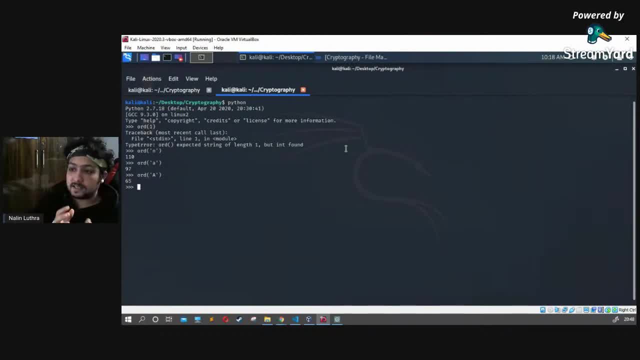 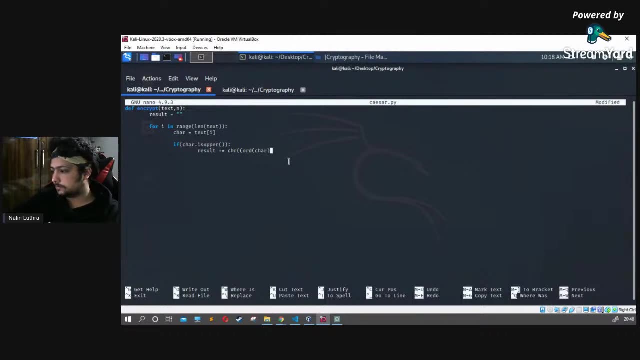 escribe values to something else. like that, like characters to escribe values. That's what ORD is used for Cool. Cool 1 for the 9. Moving forward. So we say ORD Right. So we say ORD char. Yeah, Yeah, thanks, That's right, Escribe. What, sometimes I feel I can't be a stand up comedian. 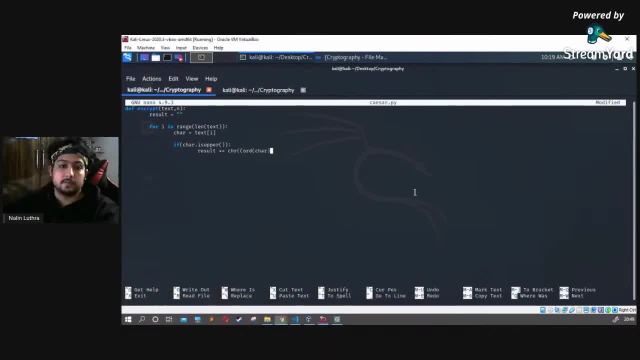 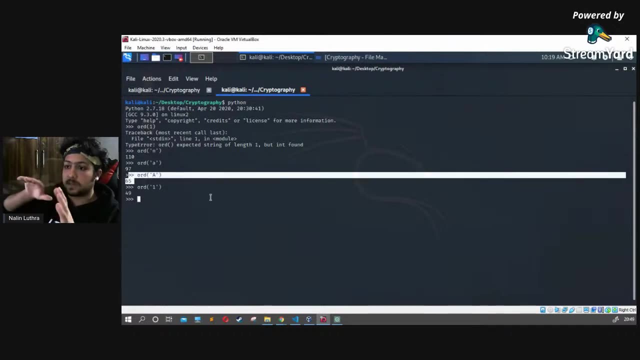 Then I just wake up from my dreams Moving forward. So we say right Plus S. So we say N minus 65. So why I'm using 65? I will tell you that. Because in case of upper like this, 65 is the basic, Like that's where it starts- 66 and so on. So we say ORD, Say B, 66. And then we go with Z, 90.. Oh, I'm looking like Z, not Z, It's Z. 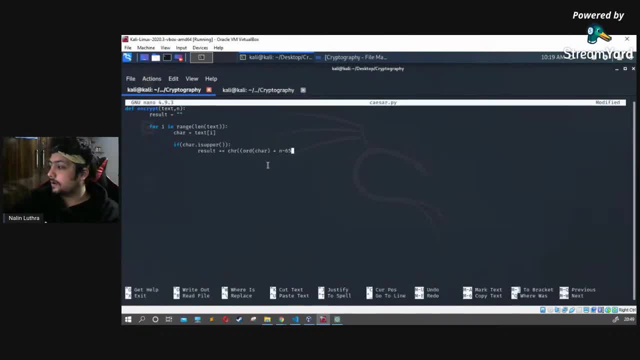 How stupid I look. Okay, Moving forward, We say: mod, Let's go with 26.. Why we're using 26?? If you don't know why we're using 26,, it's because we have 26 alphabets. That's how it is, Right. Right, So now you understand Chetan. Everything around the world is same. That's right. 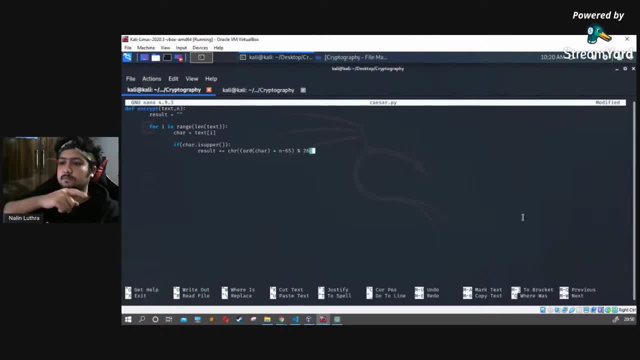 Chetan is smart, It's like Wolf Gupta. Sorry, Kidding guys, Don't take my word seriously. He's not Wolf Gupta Kidding. Okay, Moving forward now. Okay, Moving forward. We say else, Right. So Okay, We're going to say result. So if it's not upper, definitely it's lower. That's common sense, Right? So we say result plus is equal to gap, Right, CHR. 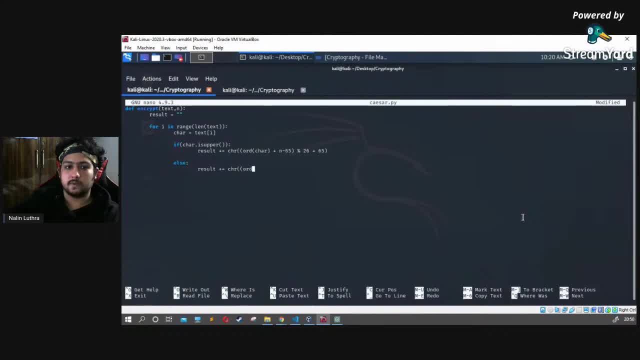 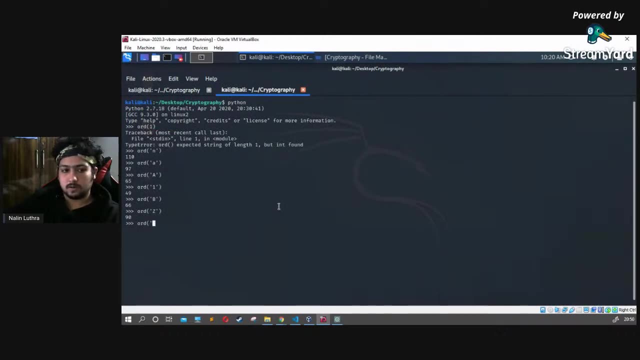 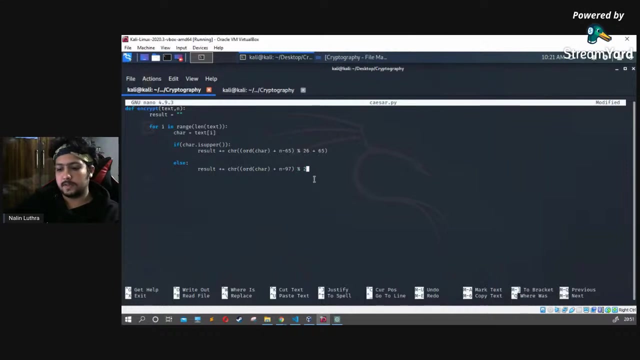 Sorry, Yeah, We call it CHR. Moving forward, We call ORD, We go with gap plus. We say N minus 97.. Cool, Now we are using N minus 97 is like this one. So we are saying ORD- I don't know Small, a Yeah, Let's go 97.. Got it. So that's why we're using 97.. Mod 26 plus What we show, 97. Cool, It's cool. 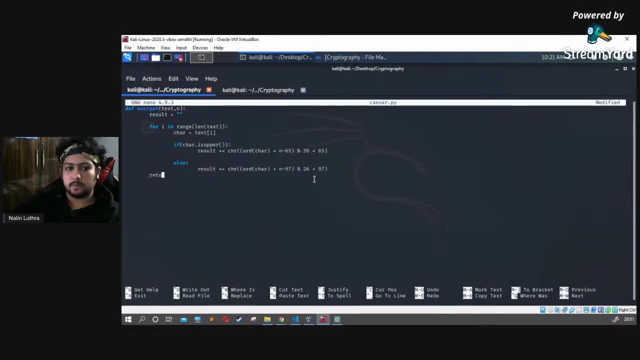 Okay, Now we say return result And we got it. So now let's start. So we have: A is equal to give me. Okay, guys, Give me something. Come on, guys, Shoot something on it. What should I encode? 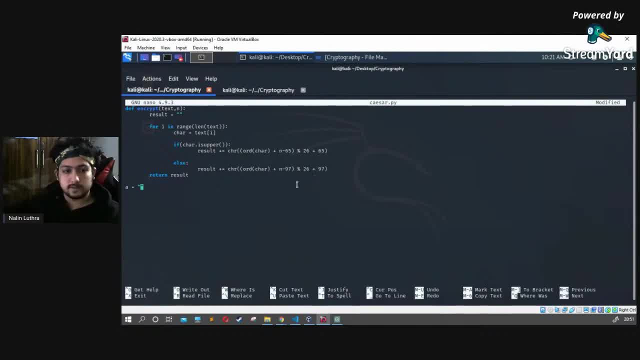 Come on, What should I encode? Can I do it? I don't know, I don't think so. I don't think, do it. so give me something, guys. what should i just encode? one one like: should i go scoring blocks, let's say coding blocks? 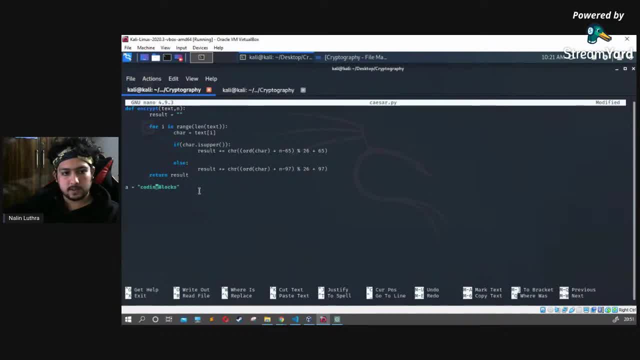 coding blocks. i will keep the b capital as well as c capital, right, so we get coding blocks, okay. okay, we see coding blocks. let's say n is equal to three. three sounds cool to me. uh, let's say print. i don't know which python i have over here. which is it? it's like python 2.7, do i? 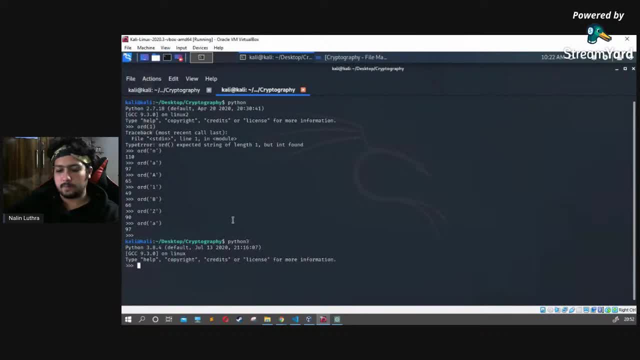 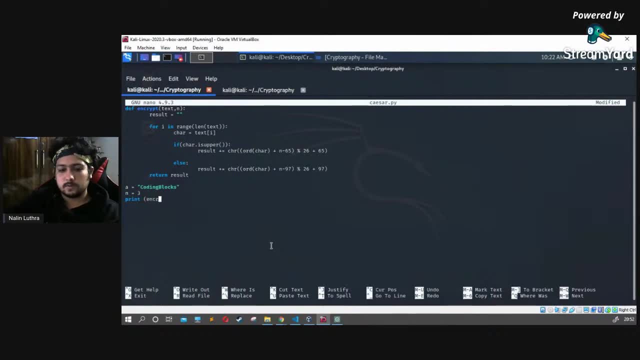 have python 3 as well on the system python 3.. now i got python 3 as well, so we will use python 3 now. so, yeah, print, i will go with encrypt and encrypt c? r y encrypt. we'll go with. encrypt a. yeah, encrypt a comma n. 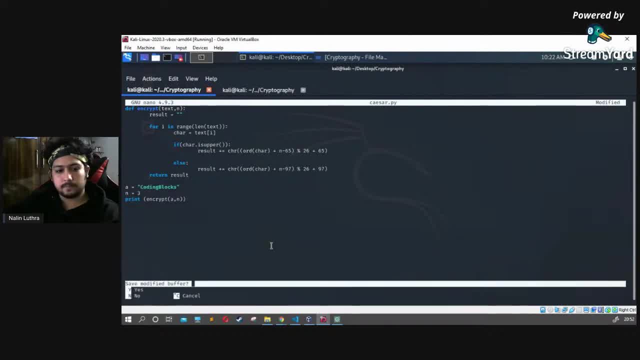 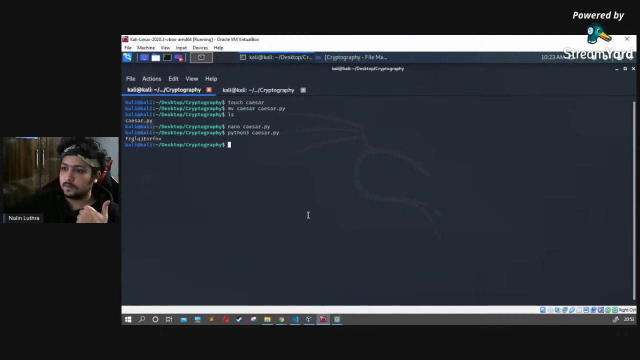 and we'll see what gets output. so we'll say, yeah, save, we press ctrl plus x and then plus y and we press enter save. don't know, let's run python 3. caesarpy got it. this is encrypted text. now answer me, how will you? 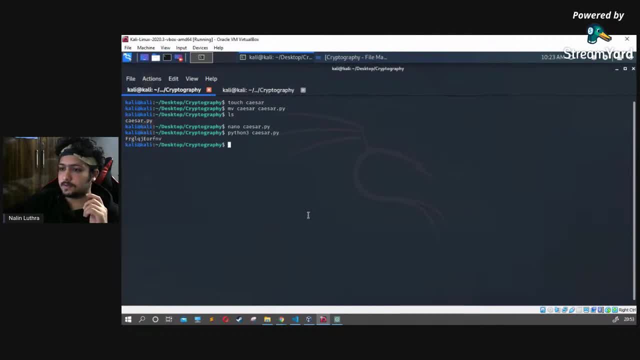 decrypt it. come on guys, think, tell me the code as quick as possible to decrypt it. i even got any idea about this one. let me copy it. come on, guys, quick, give me an answer. how will you decrypt it? come on the one. okay, oh, it's not working. now is it yet working? but now i don't. 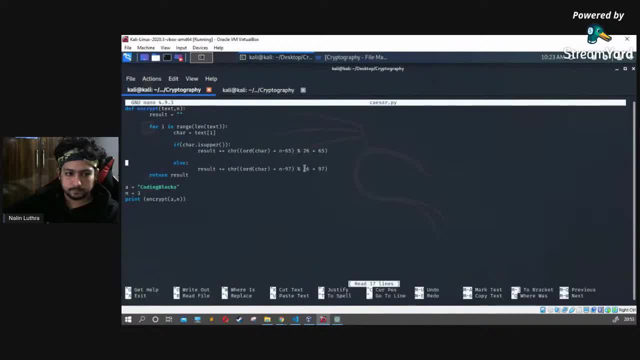 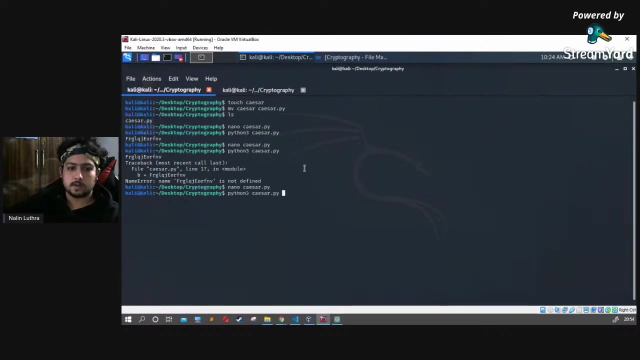 know, b is equal to this. all right, now see again, careful. r is equal to n, 26 minus n. that's simple. we say so. we say p comma r. save it, run it. okay, there's a mirror. what's there? okay, my bad, i should have done right. it's so simple. if you encrypt it using n. 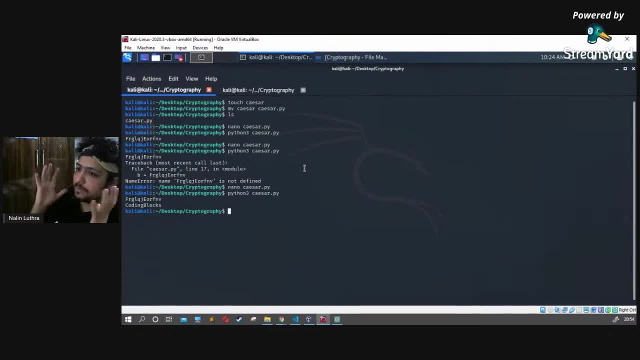 decryption is just 26 minus n wow, um. if you encrypt it using n, decryption is just 26 minus n wow. if you encrypt it using n, decryption is just 26 minus n wow, um. if you encrypt it using n, decryption is just 26 minus n wow. 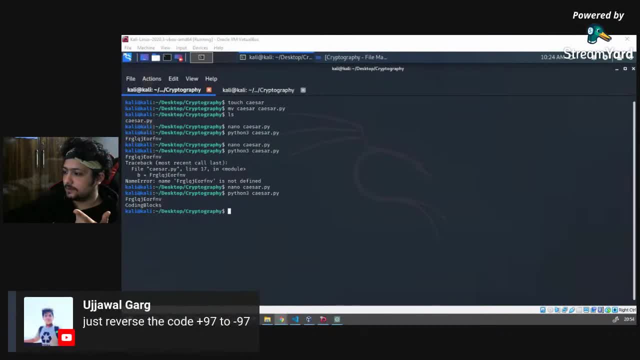 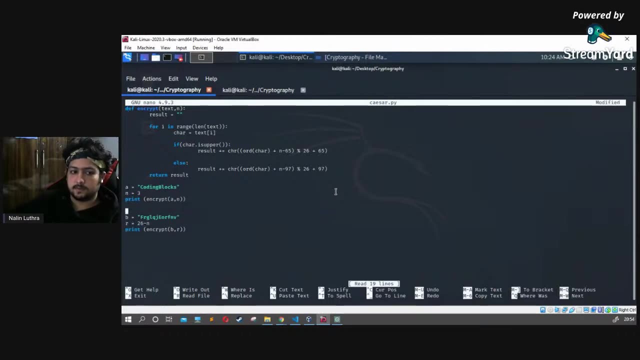 right, that's right, that's right. uh-huh, simple. okay, let me show you. this is the code for encryption, for decryption. let's say over here: yes, so so that's all. that's all. i mean, we did 26 minus n, because that was means we are reversing the. 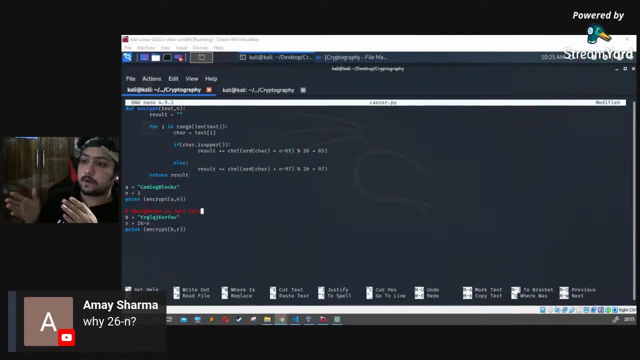 whatever we did for the encryption. that's just a reverse, like bang reversed everything. now the homework, okay, uh, okay. i'll try to explain the code once again, guys, uh, it's simple, so we took it. uh, we just odd basically means to get our square value, so we got a scribe value for all. 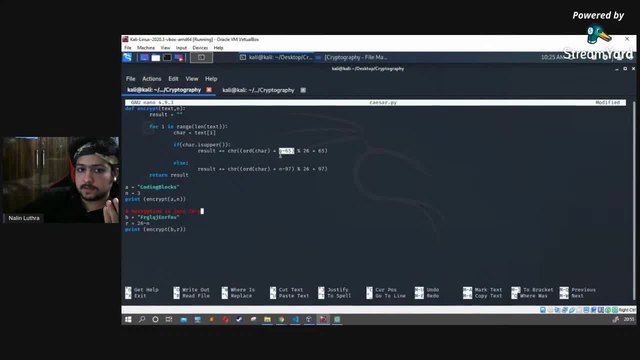 the characters one and one. then we added those vectors, depending upon what the rotation we are moving forward to, and divided by 26, right, that's how i move forward. so, uh, i don't know, today i don't have much time on this. tomorrow i will take up this code again and explain everything line by line to you. this is what. 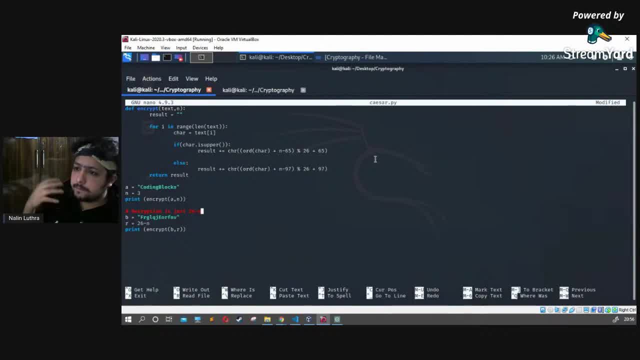 today. okay, so we will work on this code tomorrow itself and we'll improve on it. right, we'll improve on this code, okay, yeah, sure, try, go with minus one. it doesn't matter. it doesn't matter if you go with minus one either. cases, right? uh, this is your encryption for cryptography, encryption for what you're doing. 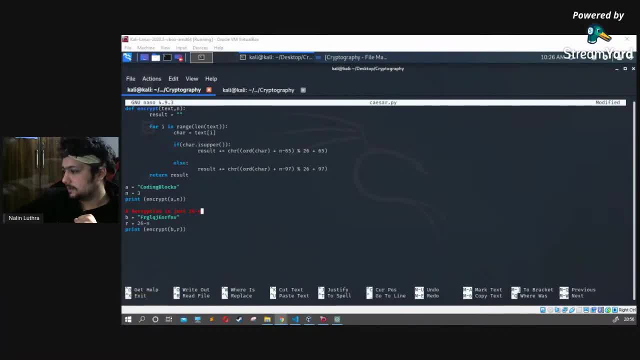 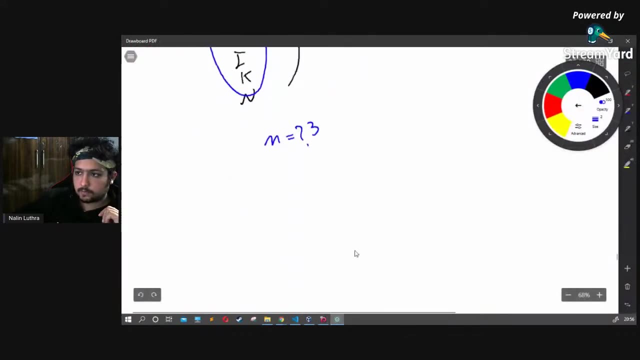 i don't know. this is a couple of encryption for c cipher, okay, okay, okay. many people got some doubts. uh, we will take up on this tomorrow's class. that's simple, don't worry about it. it's simple, i will try to explain it to you guys. so think like this: i did already explain about n. 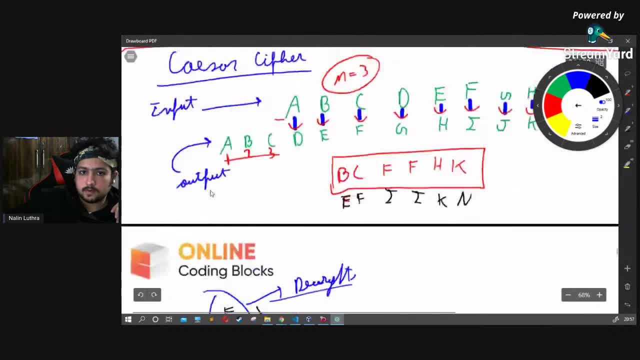 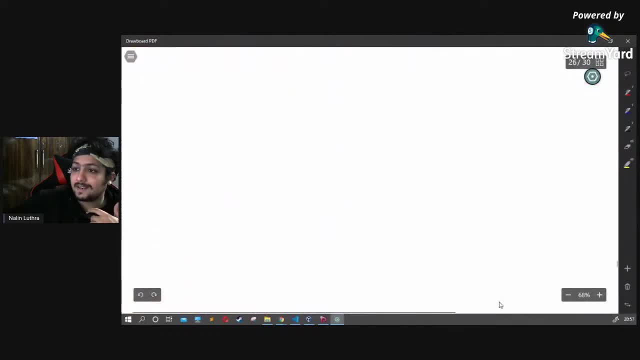 is equal to three over here, right, uh, right over here i explained written streams in that this one now. what i did was i took an ascribe value. so, for example, if i talk about small a, i got a square value 97. if i call about capital h, i got an ascribe value 63. i'm guessing that's what it is. 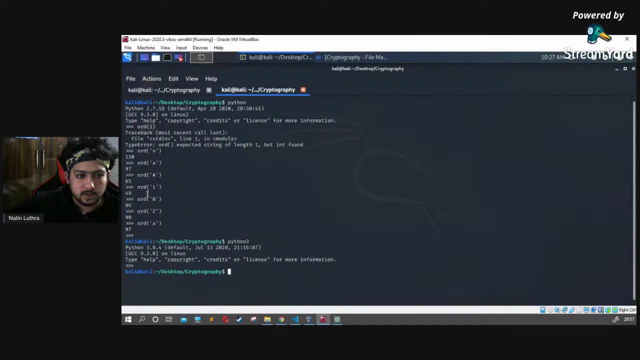 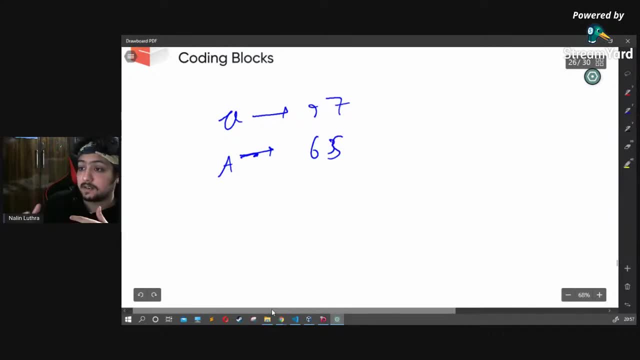 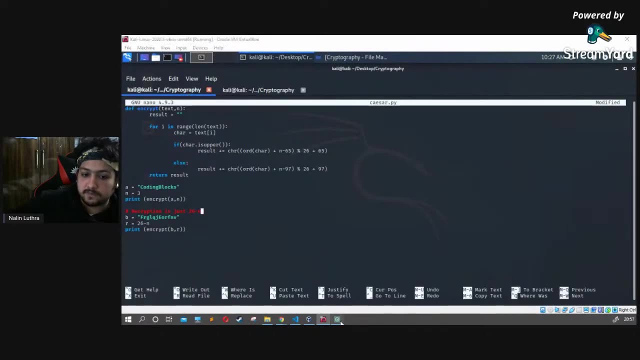 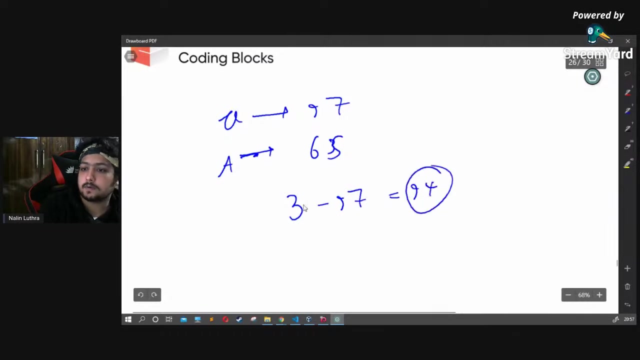 let me check it again. uh, 97 and 65, not 63, right? 65, right? so what i did? i basically spracked that amount from this. so, for example, if i look at over here, you can see over here n minus 65 means three, for example, that's three years. minus 97 is equal to 94, right? that's what i get. 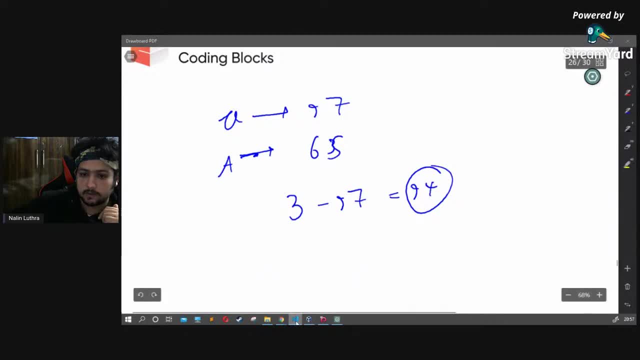 now slightly look forward to this one, uh, this one, so this one here, mod 26. so plus this. for example, i talk about 94, right? so what happens is a b 97, right? so let's say 97 plus 3 minus 97, right, you got mod. for example, i'm converting small a. 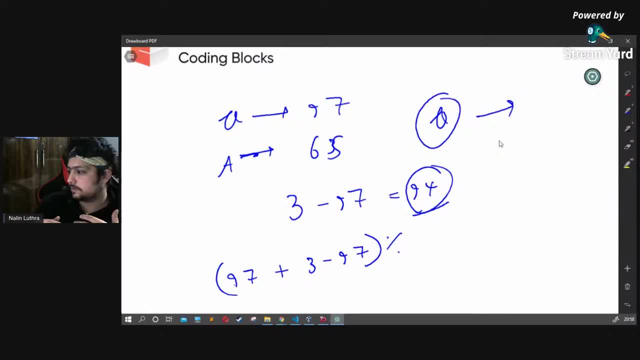 2 or into a caesar cipher, right, okay. so we take mod and we say mod 26, that's what we move forward, right, uh? what next we wrote? we wrote plus 97. okay, plus 97.. let's, let's figure this out, what it's happening. so we said 97. 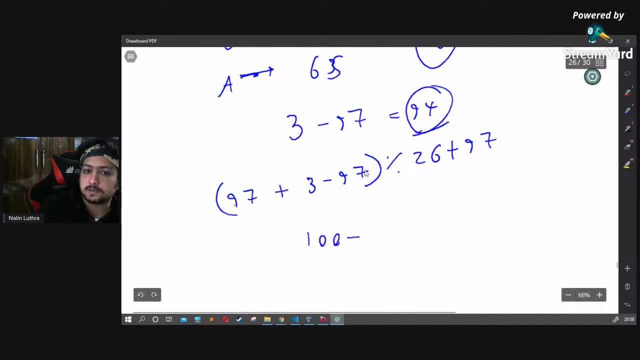 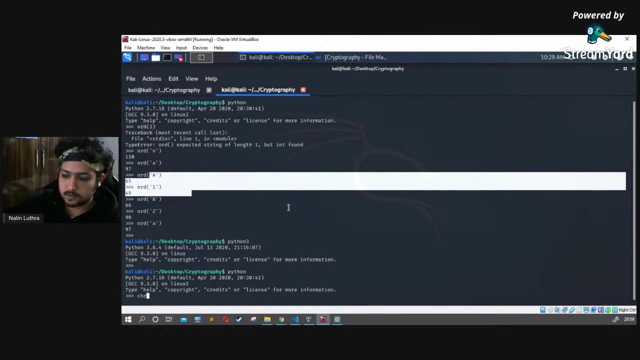 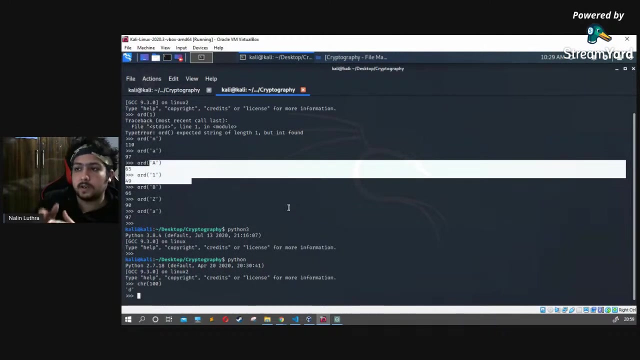 plus 3, which is 100 minus 97. which would be what? three, three mod 26 plus 97. so three more 26 is 3 plus 97. is equal to what? come on? come on guys, quick, quick, simple 100, right? so if i go over here and i write python, right, i say chr of 100, it's d, so a gets converted to. 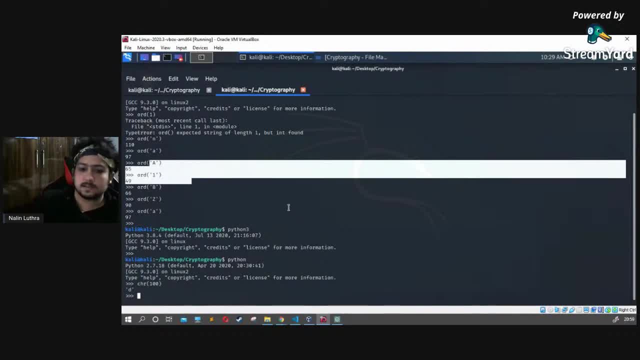 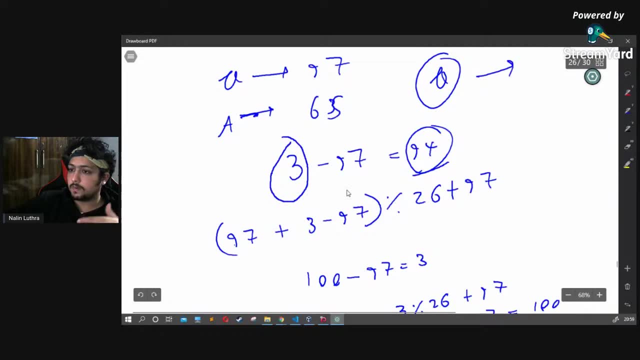 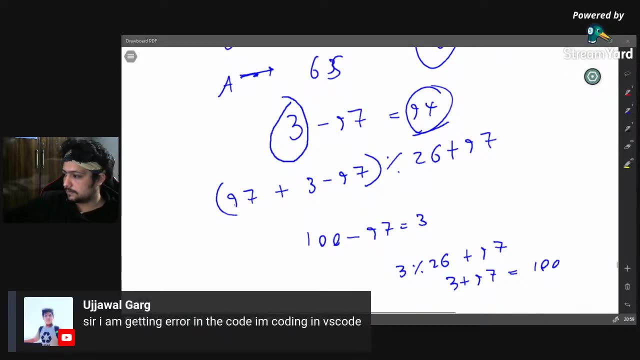 d if n is equal to 3.. how difficult is that simple right if i say n is equal to 3, right over here. so what happens is a gets converted to d, right, okay, a code is right, which? well, i don't know what area you're getting. uh, let me look better. 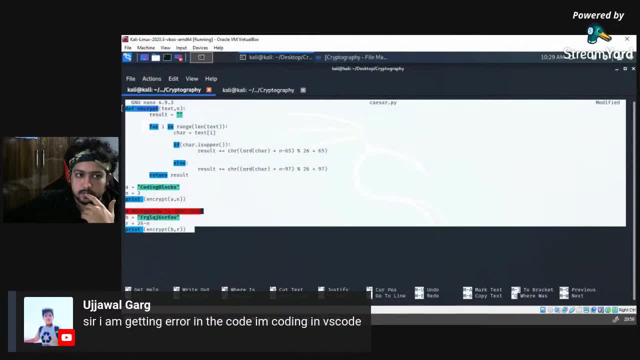 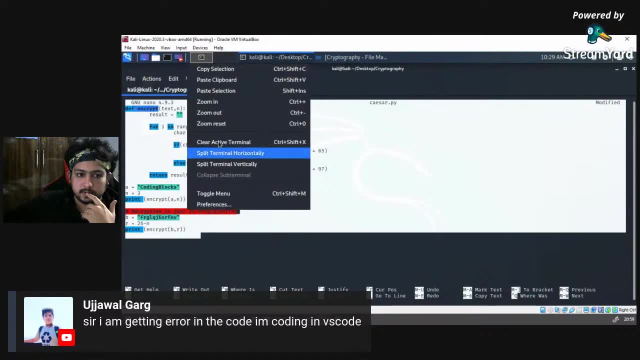 what you're getting. but this code is absolutely right. so, if you want, i can just send this code, maybe in the group itself. i don't know, is that possible copy? no, it's not, i guess i don't know. if i just copy it, i will send this code. guys, i'll set this. 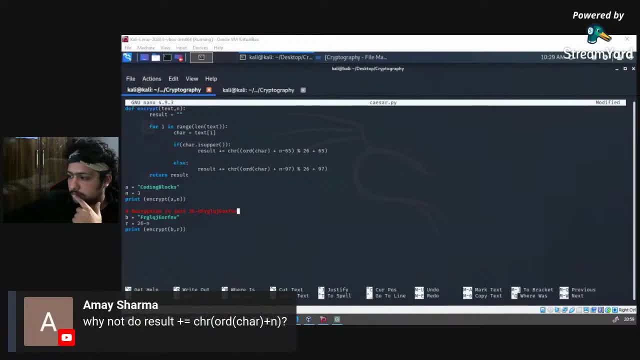 code, don't worry. okay, so we can. first of all, we can do this result, or cap plus n. can we do it? oh, we cannot. it won't give the same results. just check it out. okay now, decrypting is simple structure. what i did was i just said 26 minus n is decryption. 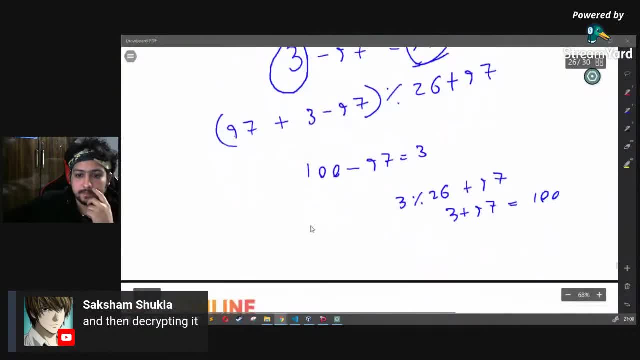 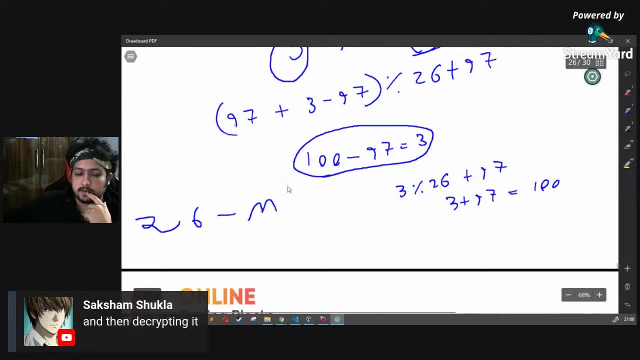 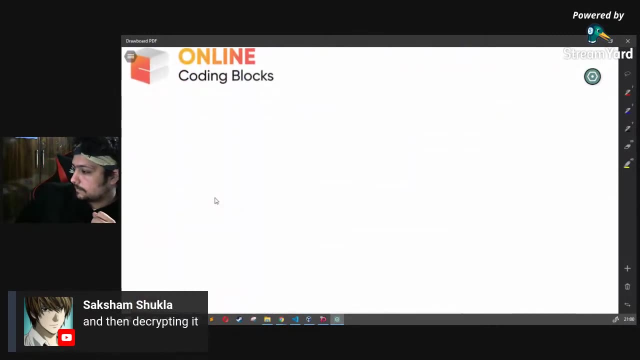 where n is encryption, simple, right, check it out. so, for example, i got three over here, right. so what i said is 26 minus n is for description. anyway, let's move forward. let's see how it goes. so about 2 to 15 pps, i guess that's how it is right. so, okay, moving forward on this one, just just. 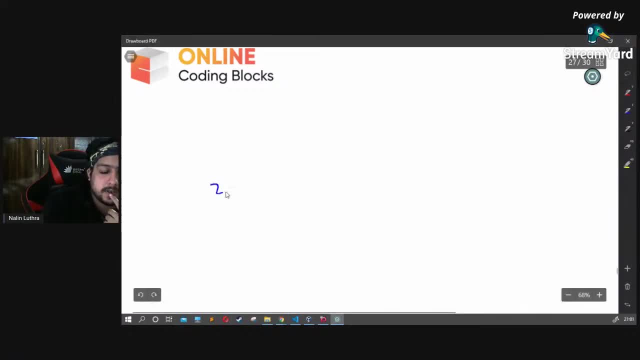 at it. if i say i got 26 minus n for decryption, how does that work in case of encryption? what i did was i said a b c. i said a b c, t e, f, right, e, t e, f, g and something so on. so what i did was: 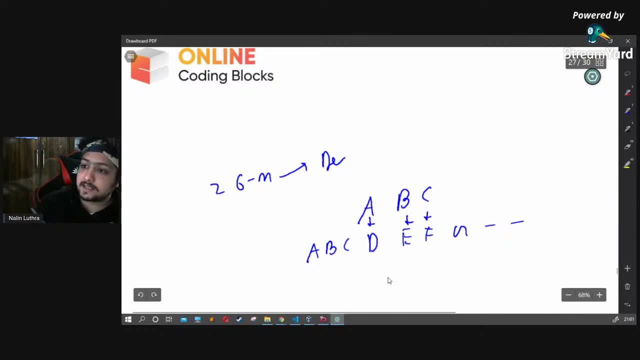 i mapped it like this. but when i mapped it like this, i said it first. now i said 26 minus n, so that means n over here is three, right, so n over here is three. now the mapping is 23. so what happens is everything gets reversed. so, for example, i say a, b, c, d, e, f, g, h, i, j, k, l, m, okay, okay, okay. 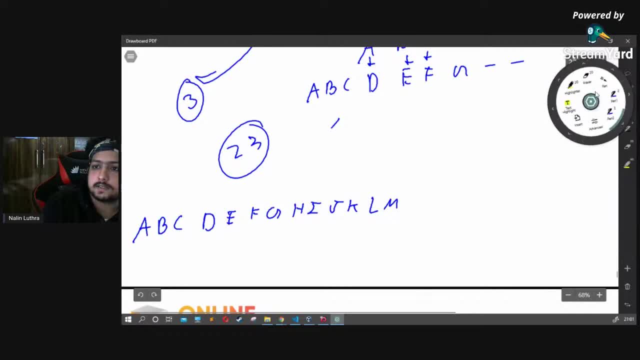 yeah, okay. so, uh, i say a, b, c, d, a, j, k, l, m, n, o, p, q, r, s, t, u, v, w, x, y, z. right now i said 23, so it should be 1, 2, 3, 4, 5, 6, 7, 8, 9, 10, 11, 12, 13, 14, 15, 16, 17, 18, 19, 20, 21, 22, 23 and 24.. 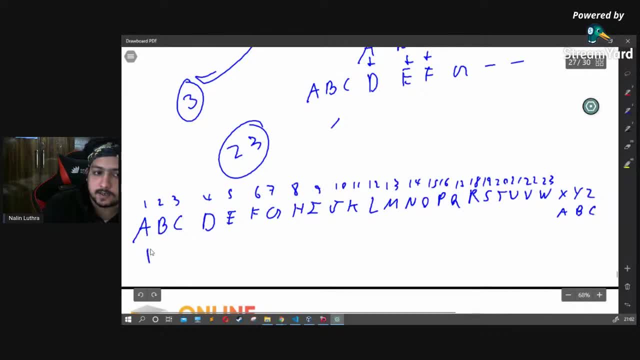 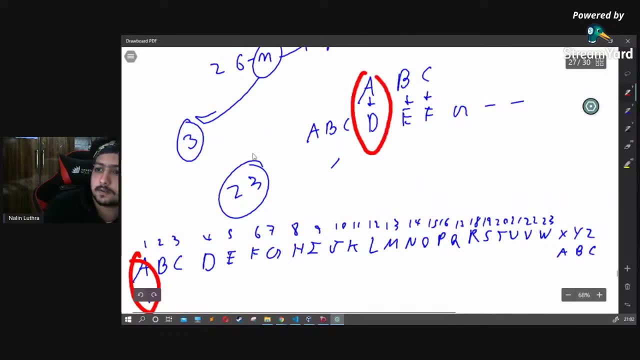 from here. we say a, b, c, d, so what happens is d maps with a right over, like this right. so when we say 26 minus n, everything matched in the reversed order. does everyone get it right, guys? does everyone get it? i think everyone did get it, so i will take the call on: everyone got it. so guys don't uh, just. 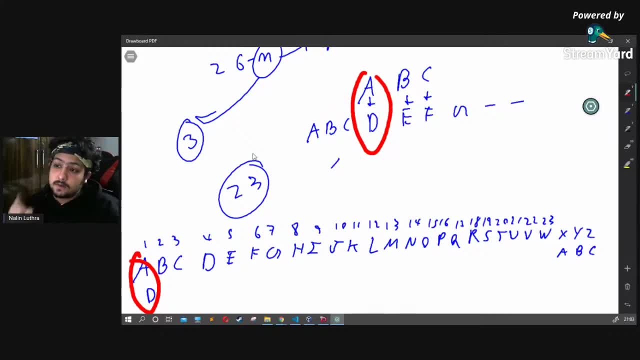 just whatever i teach you guys do practice on it. so your tomorrow's homework is: you need to find somehow- i will give you a rotational matrix right, and i won't tell you value of n. i need to come up with an output. what would the n is right.